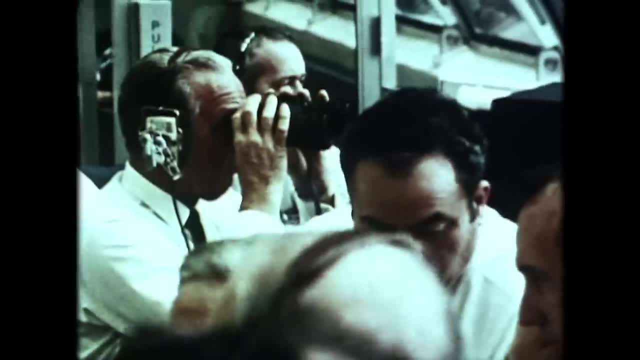 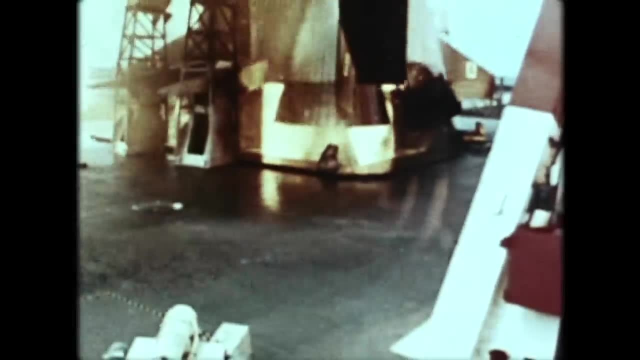 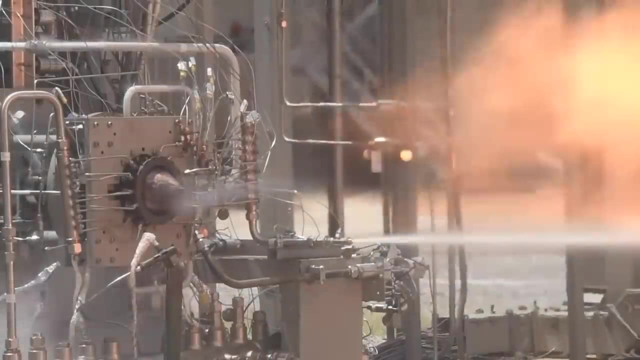 This is no ordinary rocket engine, Limited by the technology of their times. engineers and physicists have theorised this propulsion method for centuries, But the constraints of time may have just lifted with NASA's revolutionary test of this rotating detonation engine in January 2023.. 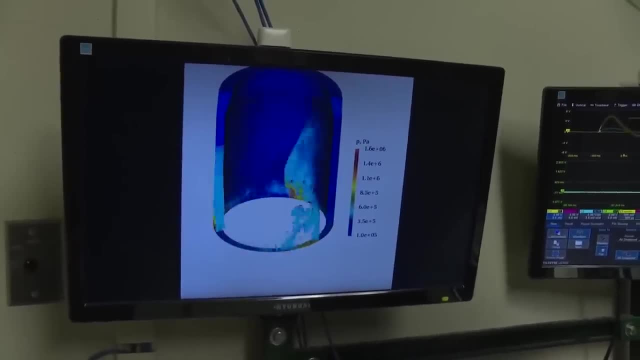 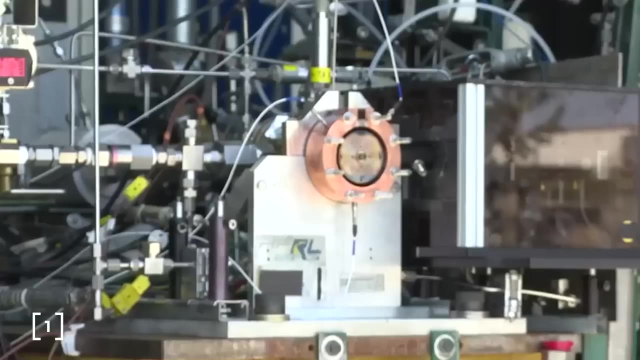 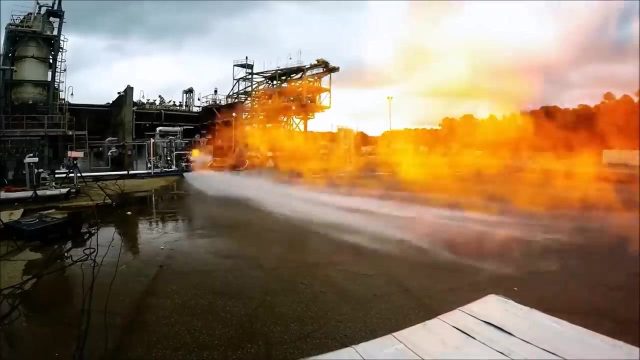 With the very latest advances in material science and computational fluid dynamics, NASA has managed to break through to test a 3D printed rocket engine that could improve fuel efficiencies of rockets by up to 5%. A 5% improvement in efficiency for a rocket is not a marginal gain. 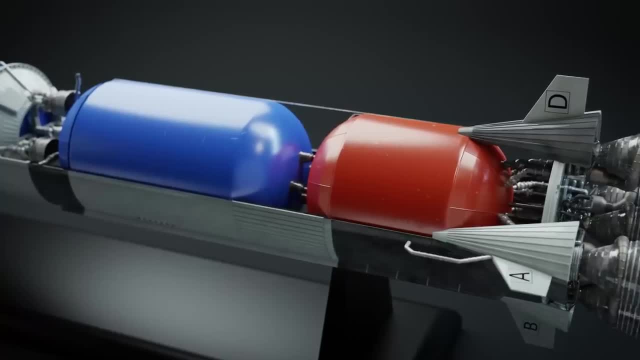 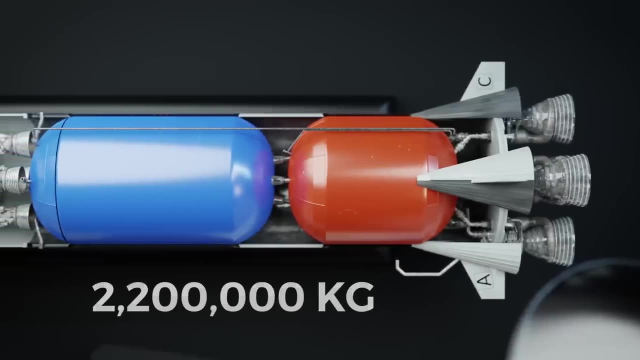 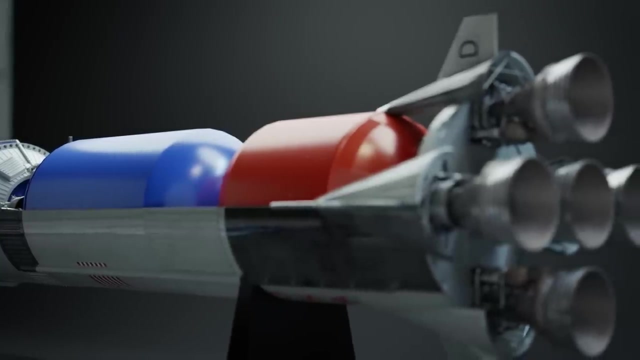 Rocket weights are dominated by fuel. The first stage Saturn V had a dry mass of 137,000 kilograms. When fully loaded with propellant, its weight was 2.2 million kilograms. The first stage was ninety-two million kilograms. A 5% increase in fuel efficiency represents a 103 tonne decrease in fuel. 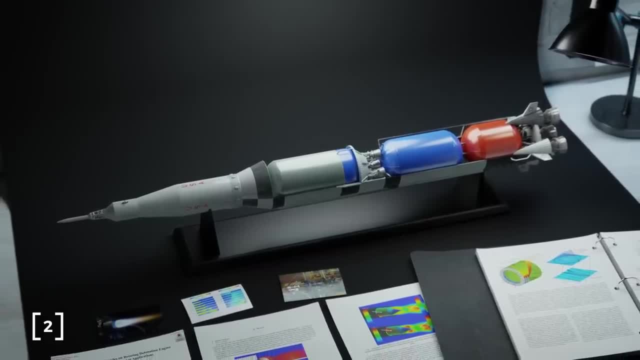 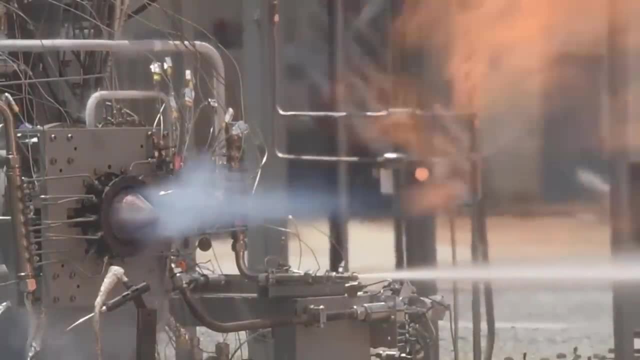 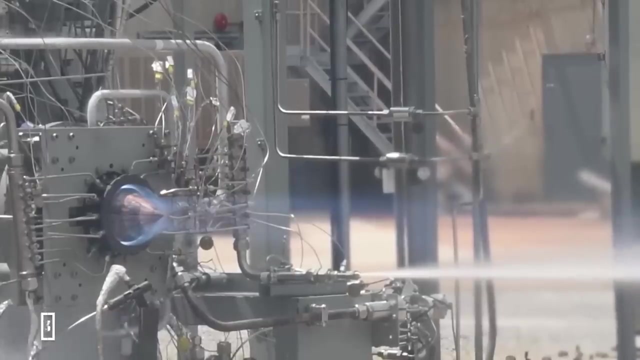 That's not far off the total dry mass of a Falcon 9 rocket. This does not just provide cost savings. It represents a drastic change in capabilities of rockets, allowing humans to launch larger payloads further into the solar system. This latest test of the technology saw the engine run 18 times, with a maximum firing duration of 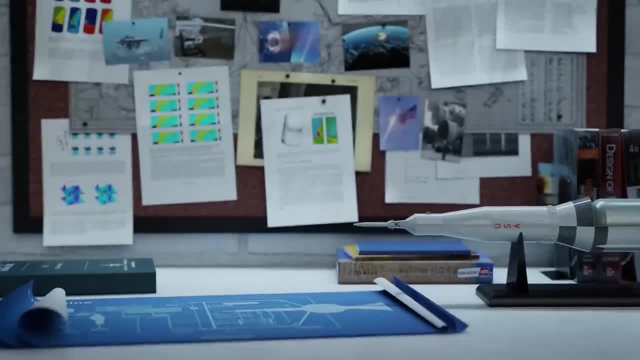 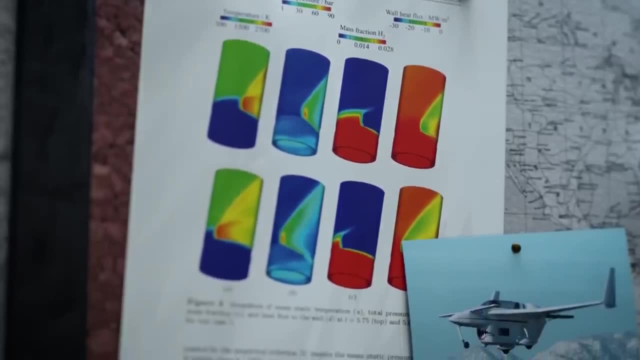 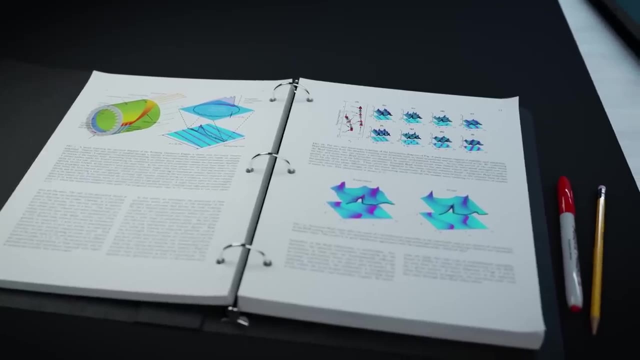 113 seconds per run. This was a test and the engine is not ready to use, But this test represents the culmination of decades of research enabled by newly developed metals and manufacturing techniques and the very latest advances in computational fluid dynamic modelling. 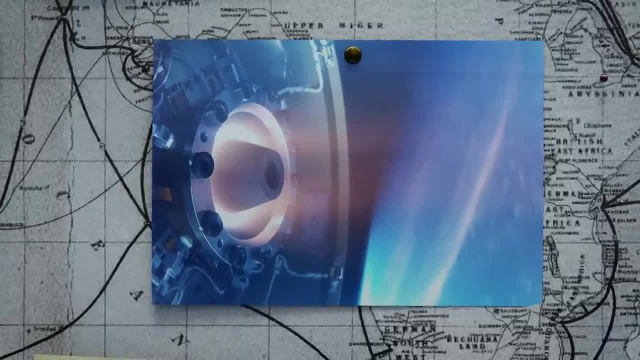 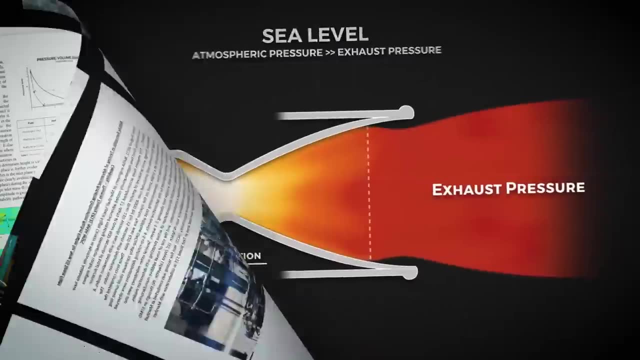 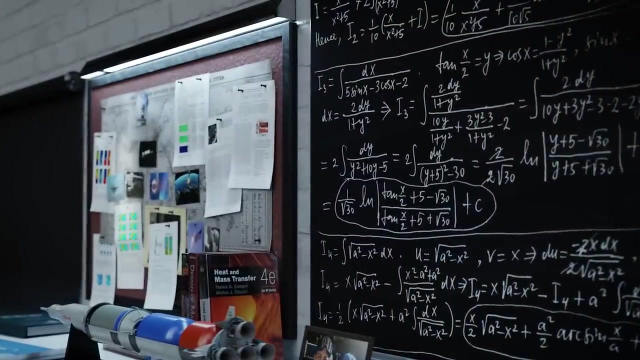 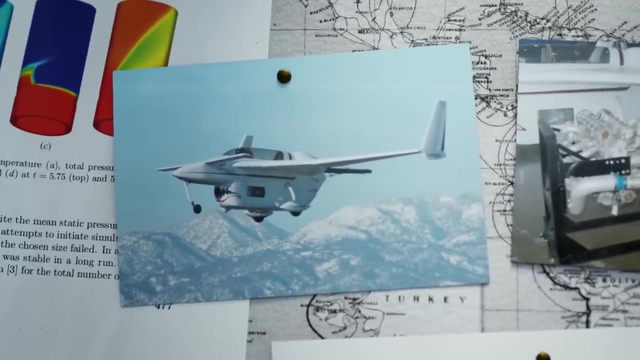 Let's delve into the science and engineering behind rotating detonation engines to see how they work. Engines Powered by Detonations. Engines powered by detonations are not a new concept. The Air Force Research Laboratory developed this highly modified Routon Long EZ, powered by four tubes, in which the detonations 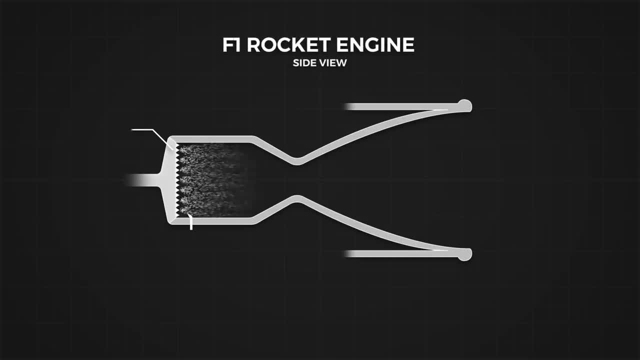 occurred. Traditional rocket engines work by mixing fuel and oxidizer using a continuous igniter. With the igniter typically located at the top of the combustion chamber, a flame front needs to travel through the fuel mixture to complete combustion. If the speed of this flame front 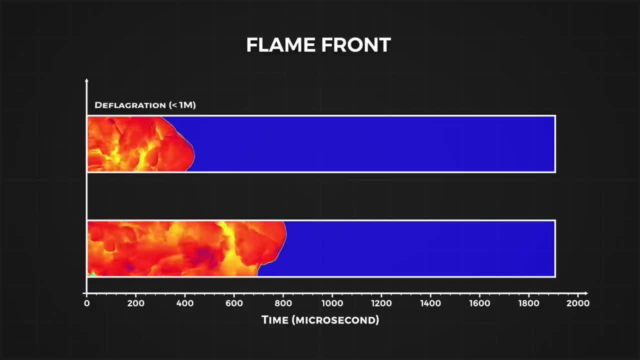 is below supersonic speed, the combustion is called deflagration. If the flame front travels through the mixture at over Mach 1, then the process is called detonation. Almost all combustion engines work with deflagrations but, as their name implies, 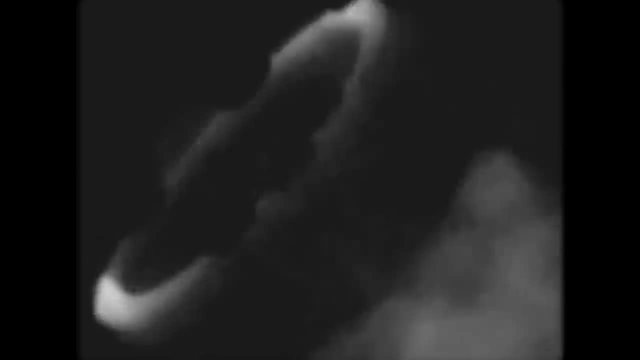 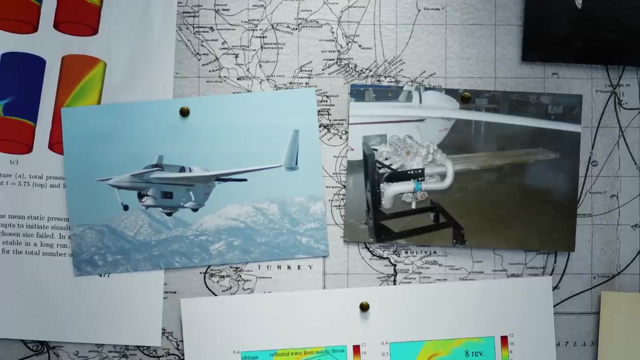 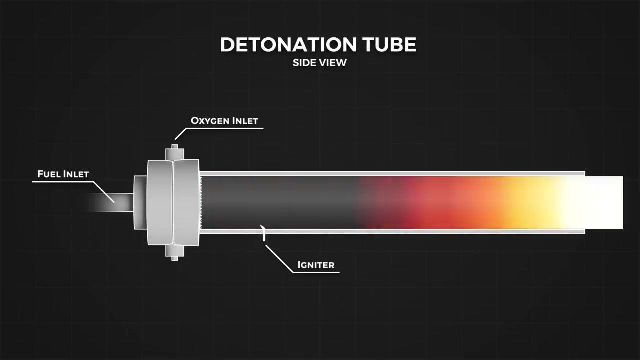 rotating detonation engines use a supersonic flame front to produce thrust and, as a result, can produce more thrust for the same time. However, this is easier said than done. The energy needed to initiate a detonation is very large and for these pulsed detonation engines used on the Air Force's test vehicle, 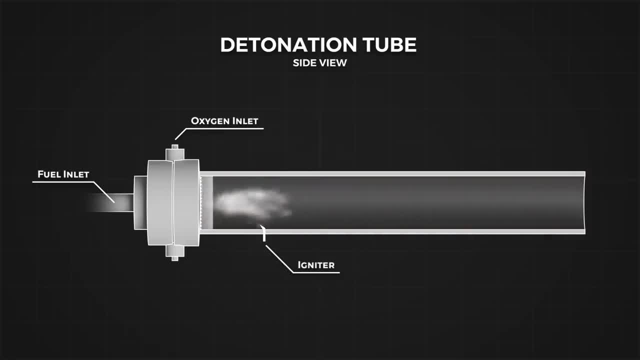 the detonations needed to happen. hundreds of times a second We can initiate a normal deflagration combustion flame front which travels through the tube and with some encouragement will transition to a detonation. But the causes of this are not totally understood and not always. 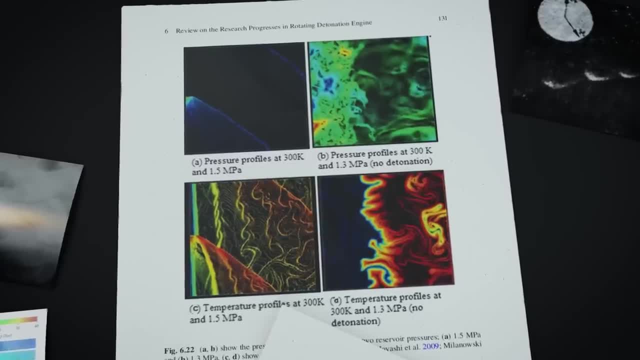 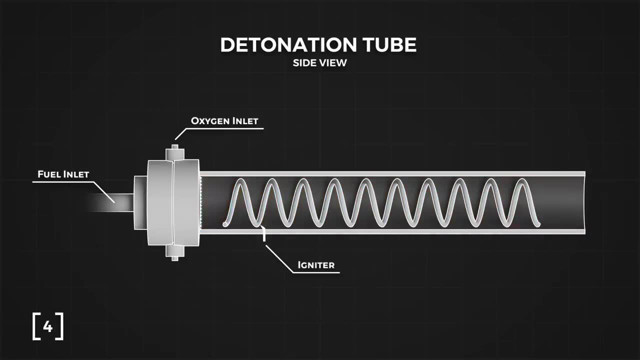 reliably repeatable. We know that detonations happen more often when the fuel is turbulent, so to create these conditions, pulsed detonation engines often include a physical barrier. One method to achieve this is by placing a spiral inside the tube. Pulsed detonations have a more 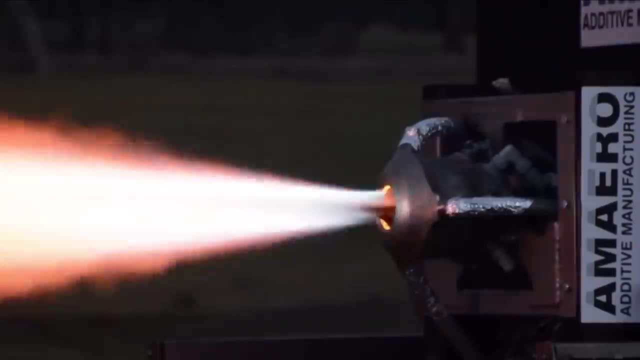 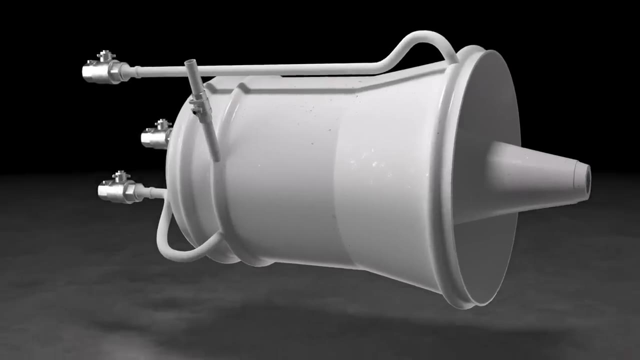 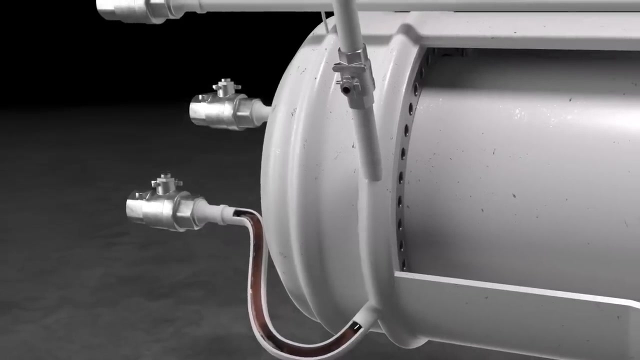 obvious problem. They don't provide constant thrust, They pulse. Rotating detonation engines are the solution to both of these problems. They consist of a ring-shaped combustion chamber. The ring starts by opening a valve at one end of the tube and letting a fuel mixture fill the tube. 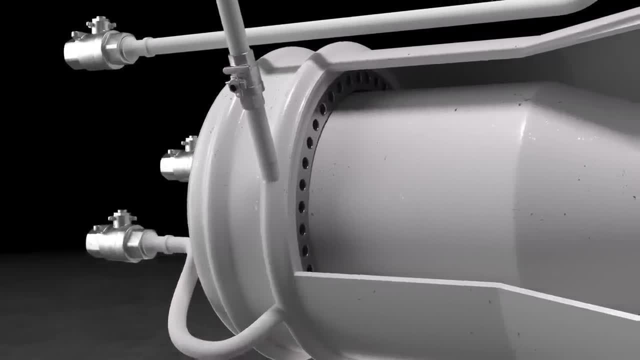 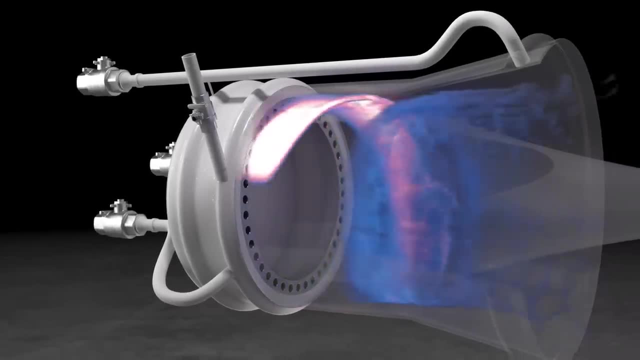 The valve closes and an ignition source at the closed section goes off and the detonation begins. A shockwave begins to travel around the circumference of the ring. This increases the pressure and temperature of the gas behind it almost instantly. This gas then expands and 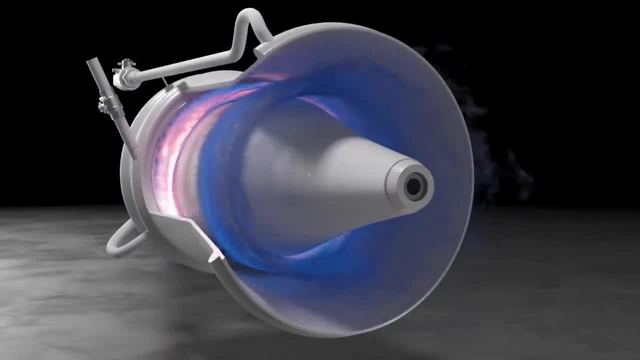 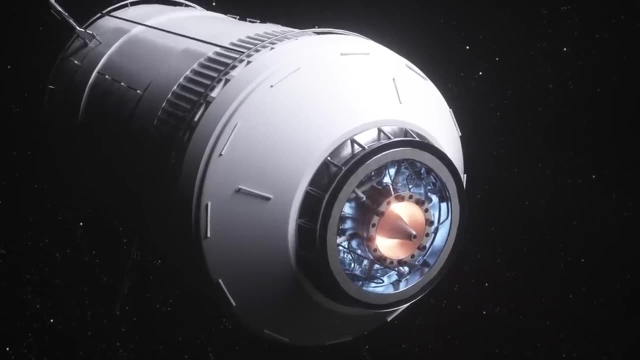 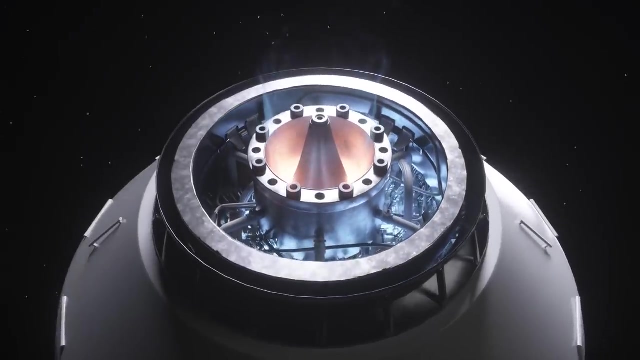 leaves the tube at extremely high velocity, creating thrust. This cycle then repeats, with the shockwave travelling in a never ending cycle. This clever arrangement solves the major problems with pulsed detonation engines by having to only set off the detonation once. It eliminates the unreliability of setting off. 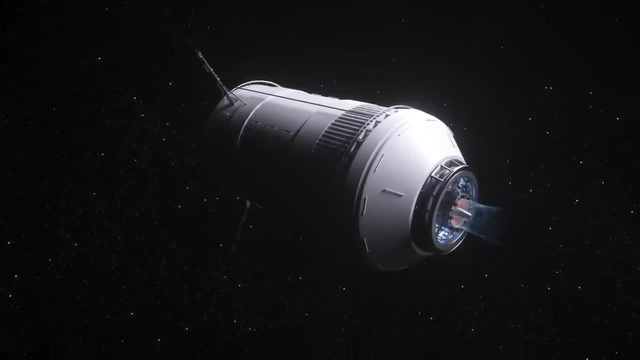 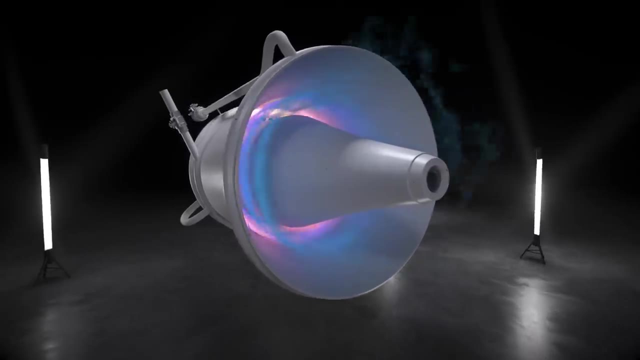 thousands of detonations. a second and its continual spiral around the combustion chamber results in consistent thrust. Keep in mind that these detonation fronts are going fast, operating at Mach 3 to 6, depending on the fuel mixture. This means the shockwave completes a full 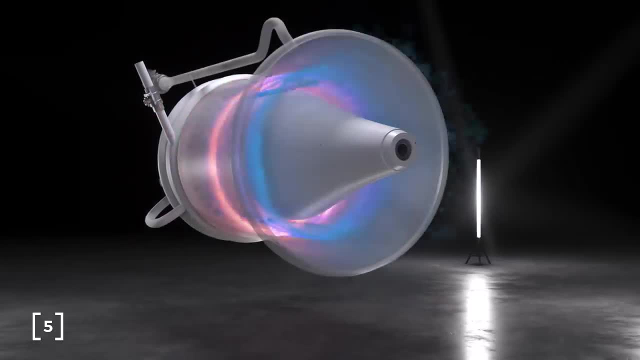 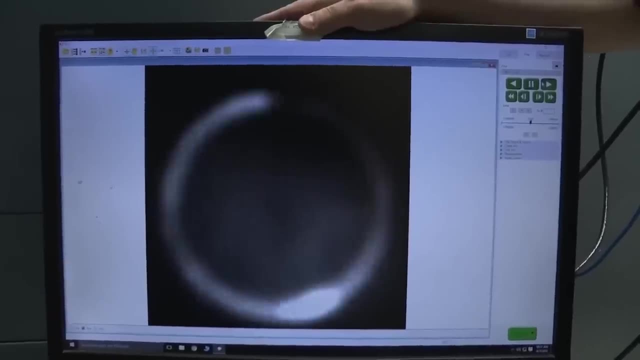 in a thousandth of a second, with operating ranges between 1 and 10 kilohertz. This is an incredibly difficult phenomenon to harness. Detonations release energy very quickly, are hard to control and are unstable by nature. In fact, for the last century of aerospace, 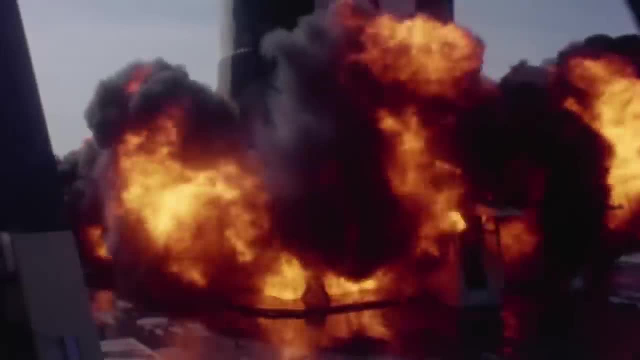 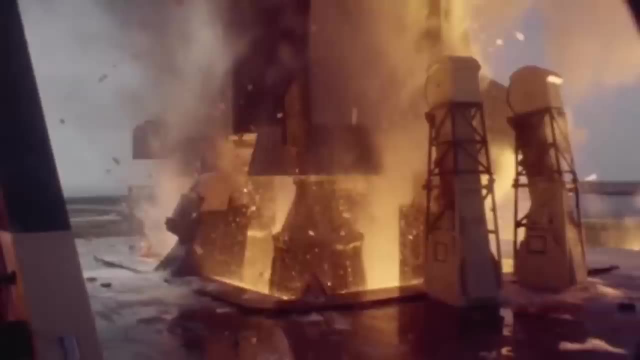 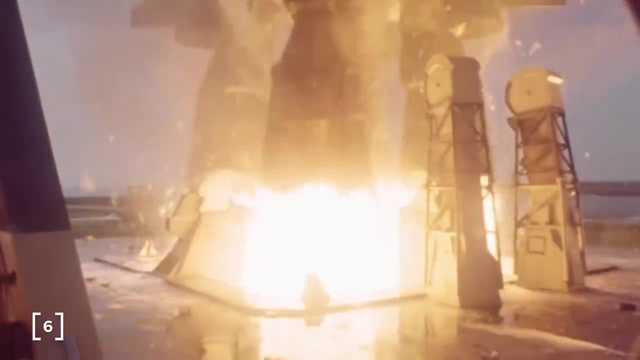 advancement. engineers have been working very hard to prevent detonations in their rocket nozzles. During the development of the F-1 engine in the Apollo program, the engineers struggled to control the F-1 engine. This was called thermodynamic instabilities. These were, in fact, detonations. 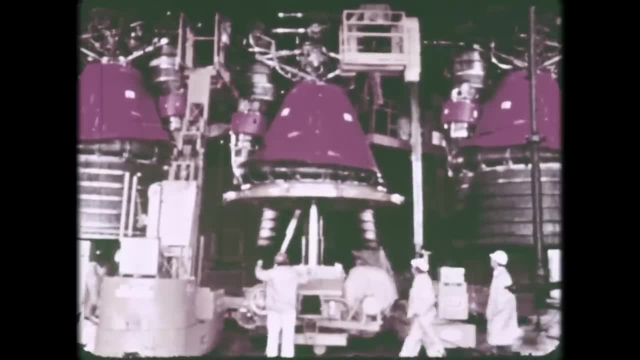 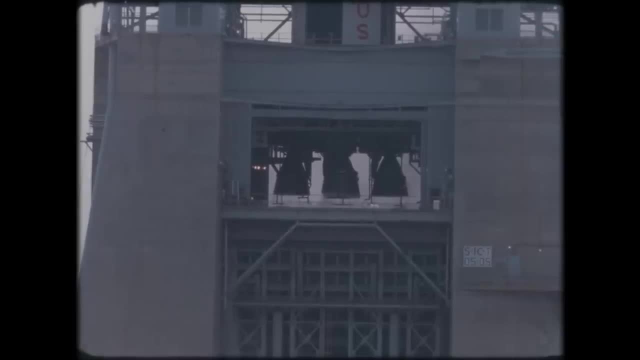 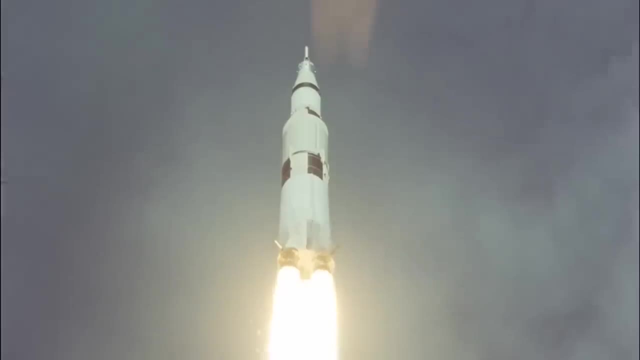 that were destroying the engine. On June 28th 1962, these combustion instabilities caused an engine to be completely destroyed during testing. This problem was plaguing the engineers of the Saturn V and it is arguably the greatest challenge they faced in scaling this monstrous rocket to. 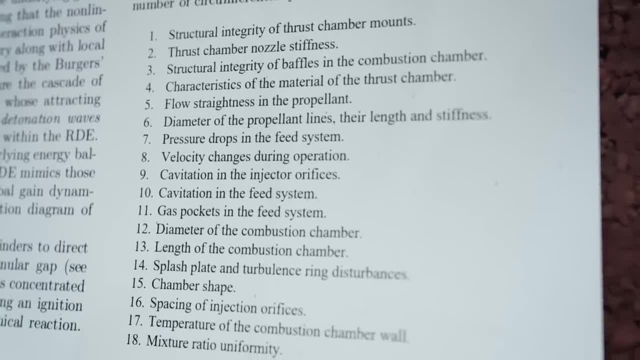 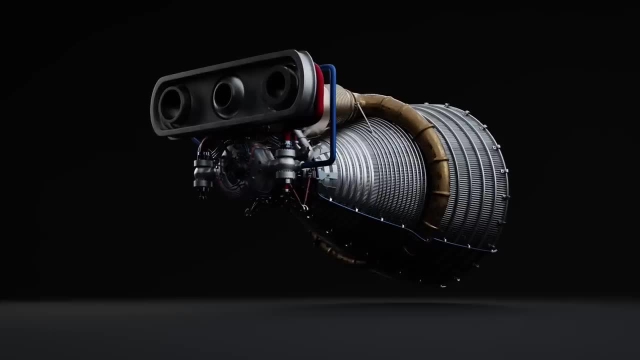 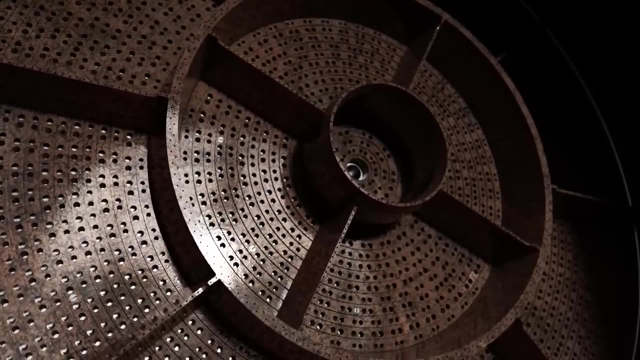 reach the moon. A list of 18 potential sources for the instability was made. This was an incredibly complex and dynamic problem. One method to reduce instabilities and to prevent pressure waves from amplifying off the side walls like a sound wave was to install baffles that separated the combustion chamber radially. 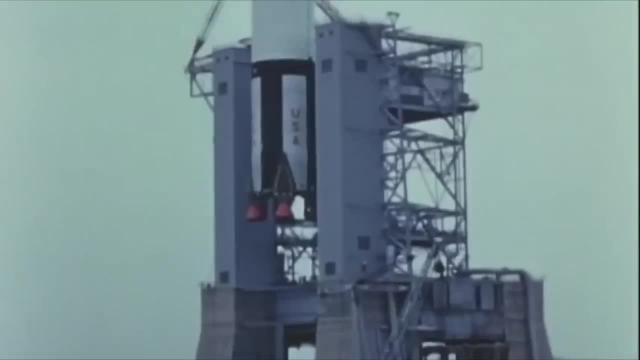 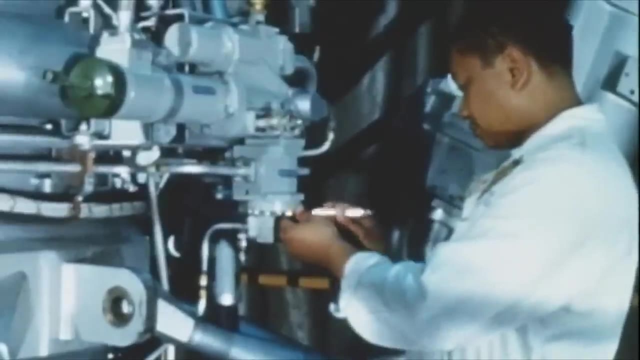 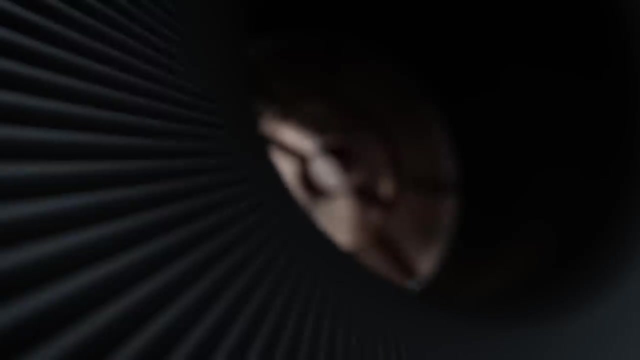 Several iterations of baffles were designed, but with no computational method available, the engineers of the F-1 engine turned to the next best practical method. They set off tiny bombs inside the combustion chamber during operation to quickly induce small combustion instabilities. This condition was called the n slider the combustion chamber. 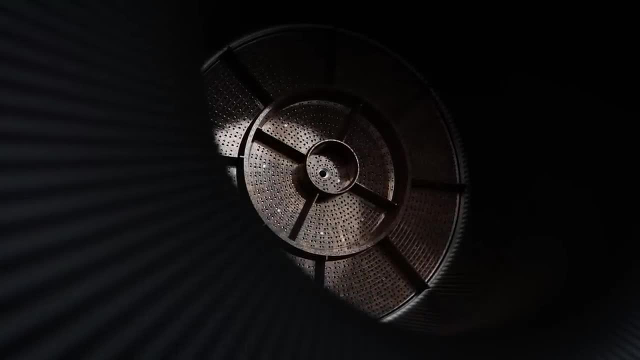 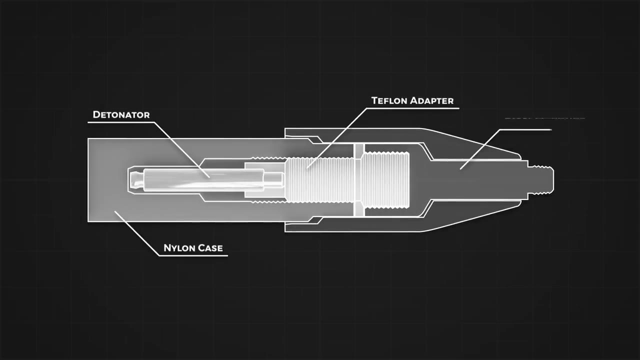 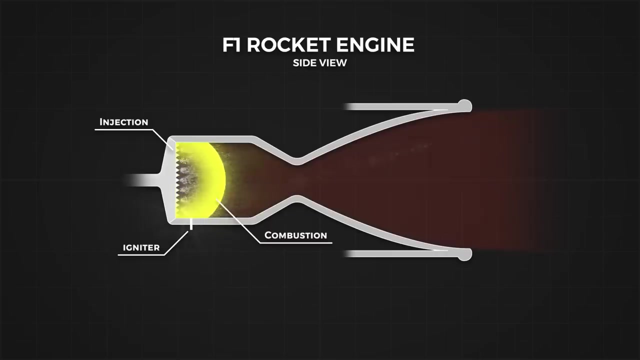 bomb was attached to the injector plate, with the detonator inside this combustion zone. The detonator was enclosed in nylon that would ablate away in the heat of combustion over time, allowing the engine to reach full operation before detonation, Resulting in a pressure wave that travelled through the engine, just as a combustion instability would. 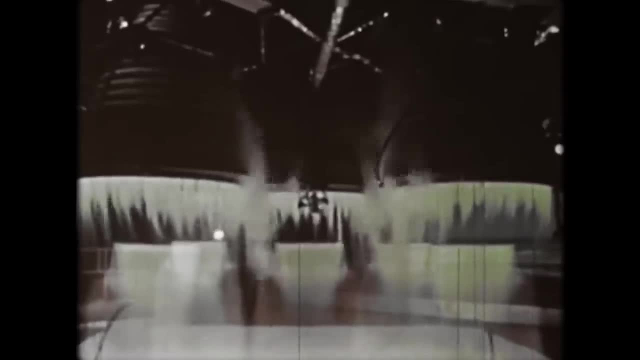 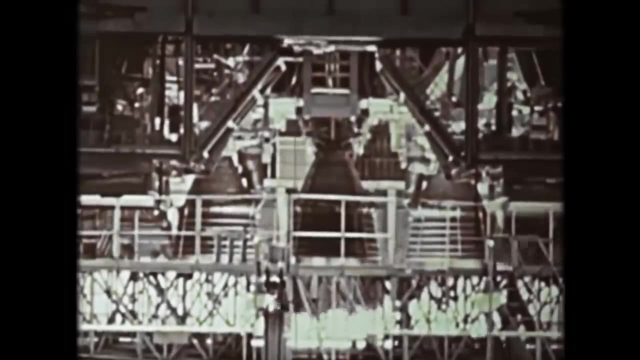 The engineers could test the effectiveness of this new baffle design by timing how long it took for no proper combustion to start. This would result in a mechanical downfall of the engine. as if the normal operation to resume after the detonation, These baffles effectively acted as acoustic dampeners, like the foam wedges we place in. 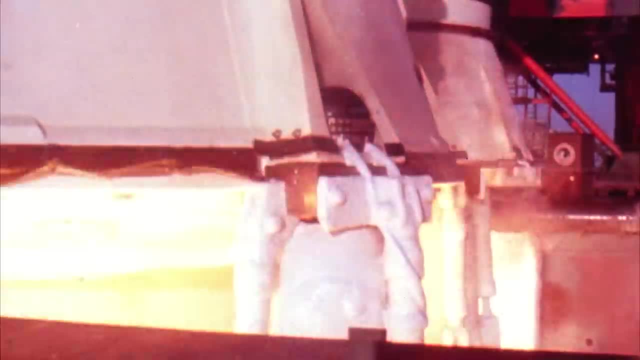 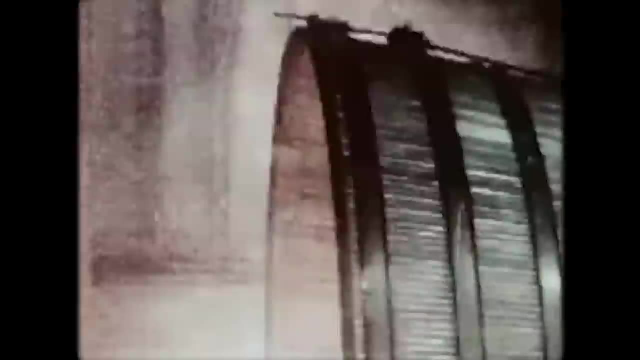 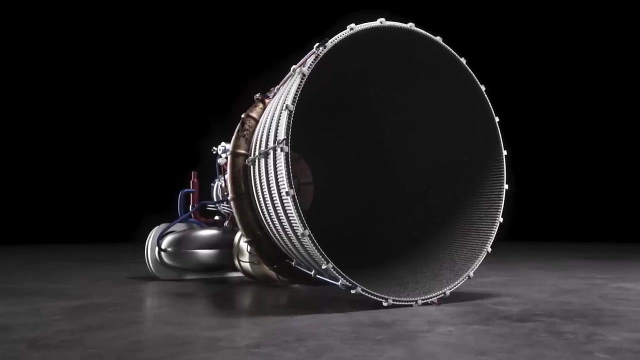 sound treated rooms. For decades, engineers have been working to prevent uncontrollable dynamic detonations, But engineers and scientists are stubborn kinds of people When they hear uncontrollable, all they hear is not yet controlled, And rotating detonation engines effectively used the exact phenomenon that these baffles. 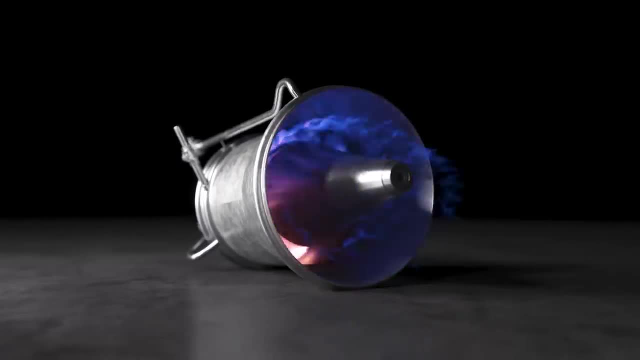 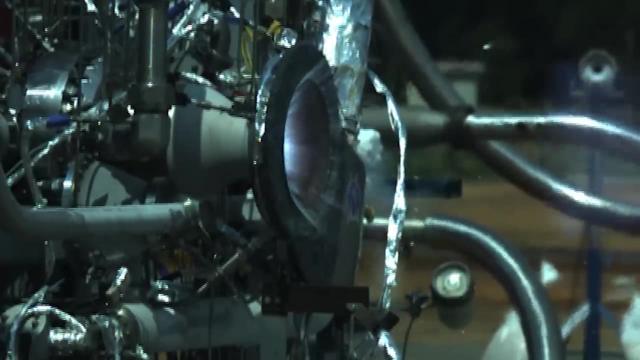 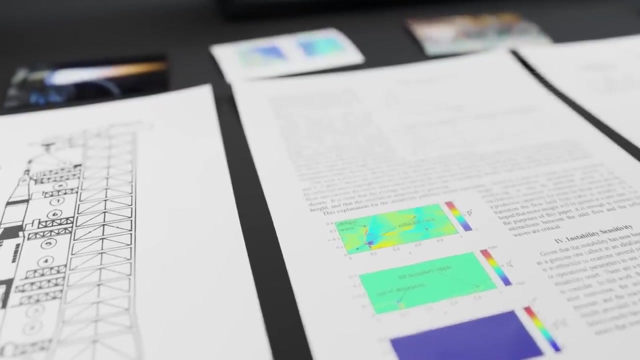 were trying to prevent Allowing a shockwave to travel tangentially around a ring shaped combustion chamber. The appeal of using detonations as a combustion and propulsion mechanism is precisely what makes them dangerous: their quick release of energy. We can visualise the amount of energy we can extract by comparing the combustion cycle. 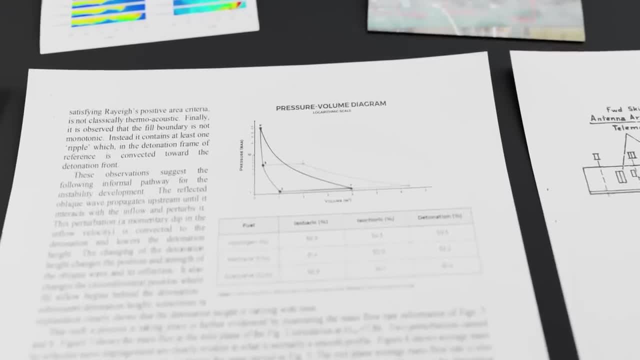 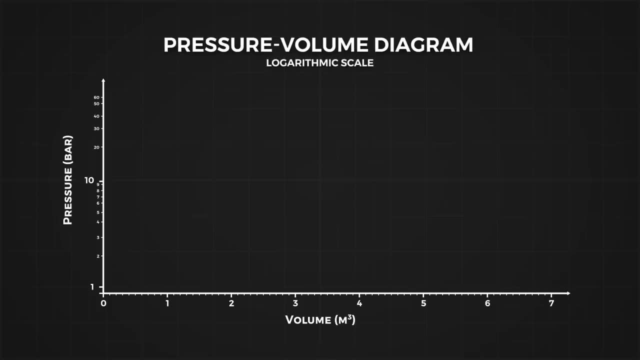 of a hypothetical detonation engine and a normal gas turbine engine on a pressure volume chart. This chart simply plots the pressure and force. This is the volume of air as it travels through an engine. In a gas turbine, the air enters the engine at this pressure and volume. 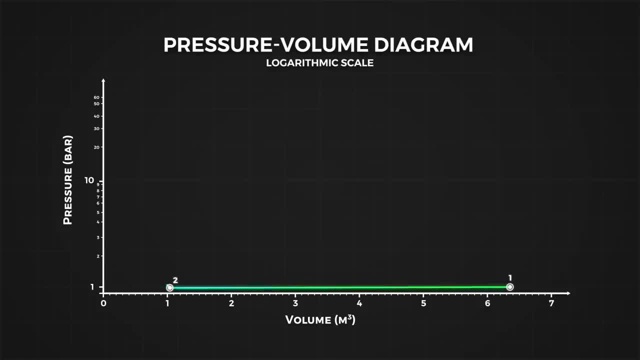 A compressor decreases the volume at a constant pressure. It then moves to a combustor, where heat is added at a constant pressure. Then the gas passes through a turbine as it expands until it reaches its initial condition again. The energy we extracted can be found by finding the area enclosed by these curves. 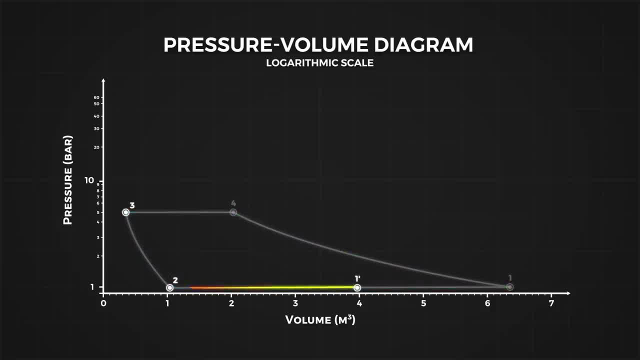 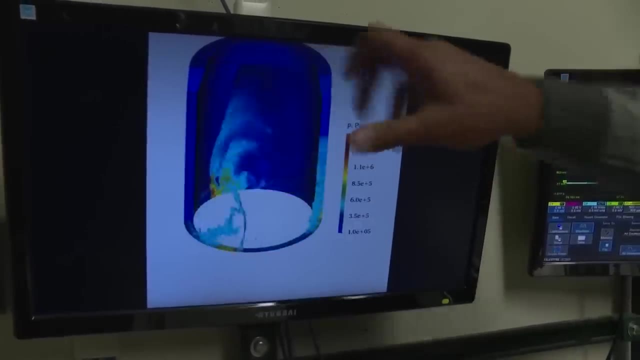 In a detonation cycle, we skip the combustor stage. Instead, the detonation wave increases the pressure of the gas almost instantly, spiking it much higher. This creates a much larger area inside the curves. The theoretical differences in thermodynamic efficiencies using this analysis method are: 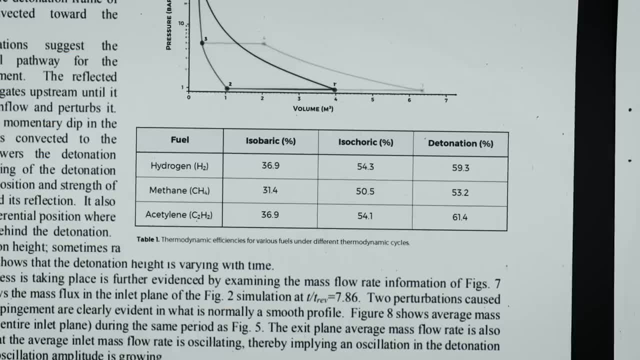 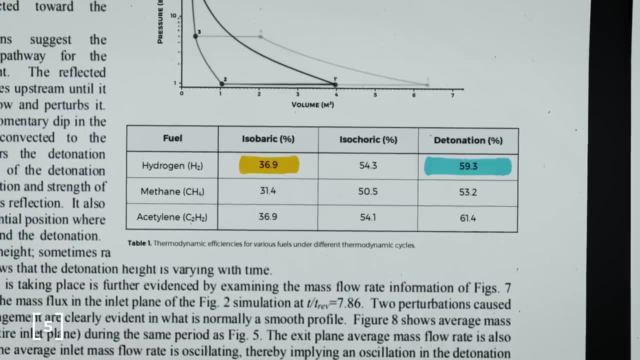 immense Using hydrogen as our gas. a gas turbine engine has a thermodynamic efficiency of 36.9%, while a detonation engine has a thermodynamic efficiency of 59%. The gas turbine engine has a thermodynamic efficiency of 36.9%, while a detonation engine 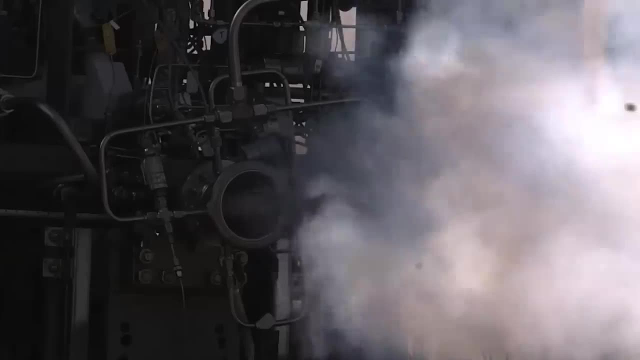 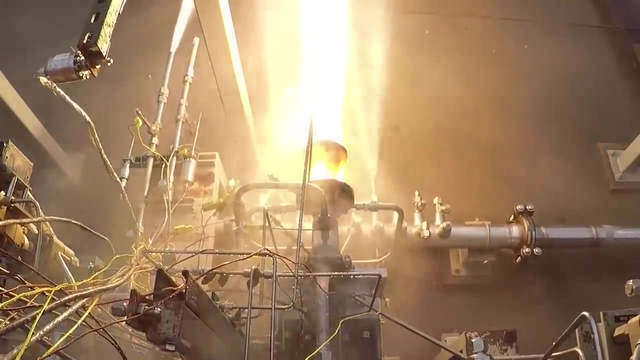 has a thermodynamic efficiency of 59%. The gas turbine engine has a thermodynamic efficiency of 59.3%. Simply, this means more energy is extracted from the same amount of fuel. However, an increase in energy yield is of no use to us if we can't control it or 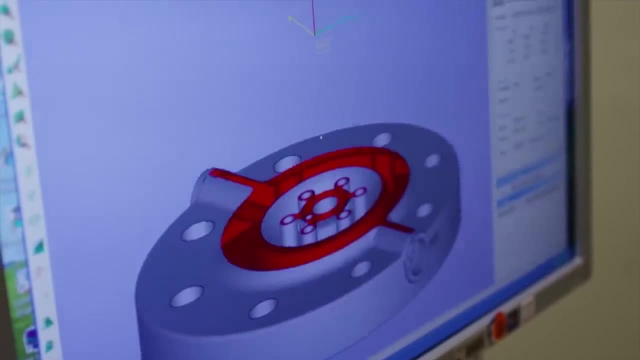 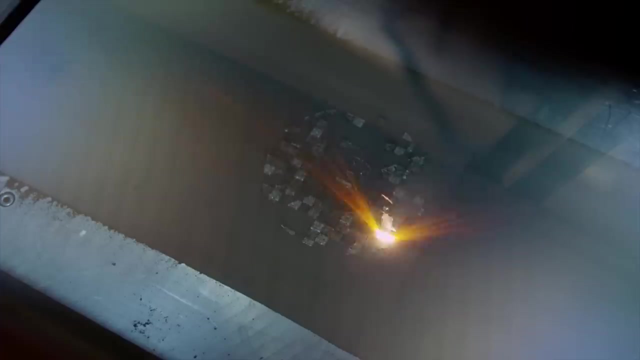 it simply destroys our engine. To harness this energy, we needed to develop new materials and manufacturing techniques. This is where a new material specially developed for metallic 3D printing comes into play: GR COP 42. A NASA developed alloy made up of niobium, chromium and lithium. 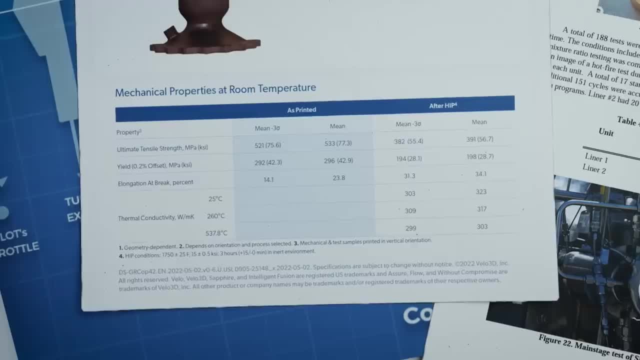 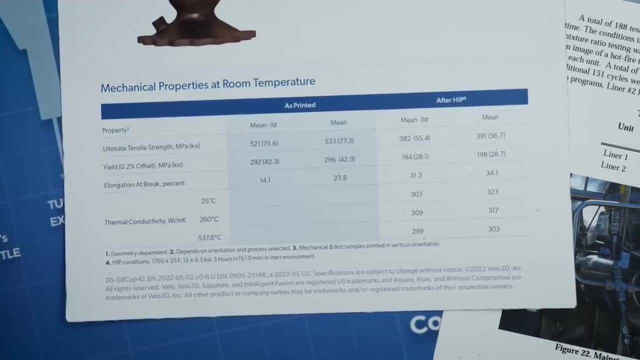 It is the most expensive alloy in the world. It is the most expensive alloy in the world. It has a high strength metal alloy specially formulated to not only have a very high melting point but a very high thermal conductivity, Meaning it takes more energy to melt it and it conducts the energy away more efficiently. 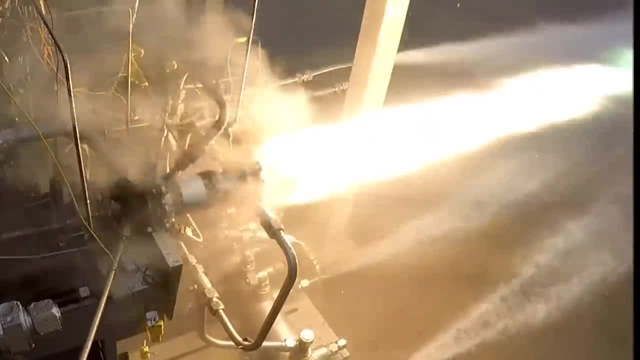 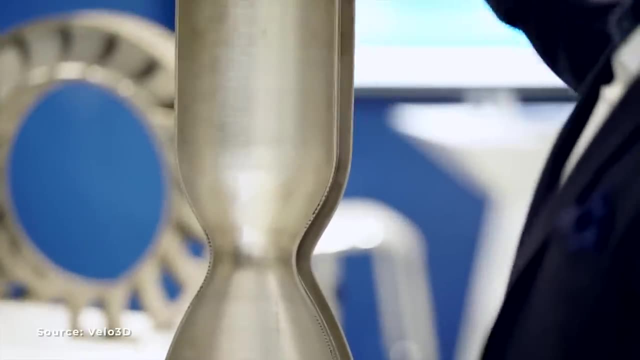 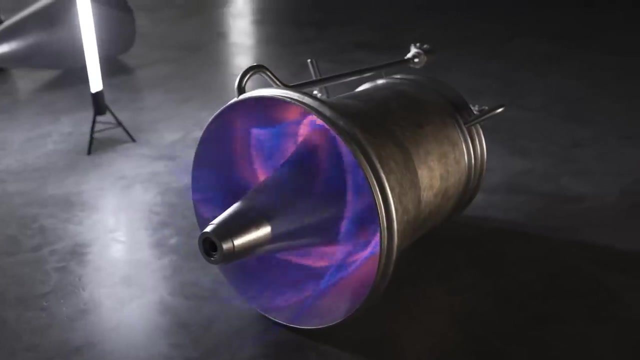 to prevent itself from melting And critically. NASA has more recently developed a method of using it in metallic 3D printing Meaning. we can create incredibly complex geometries with this new age material. Maintaining this reaction is incredibly difficult. The shockwave by nature is travelling incredibly fast and causes rapid changes of temperature. 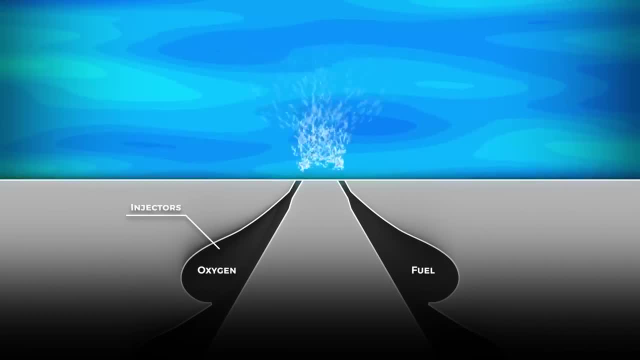 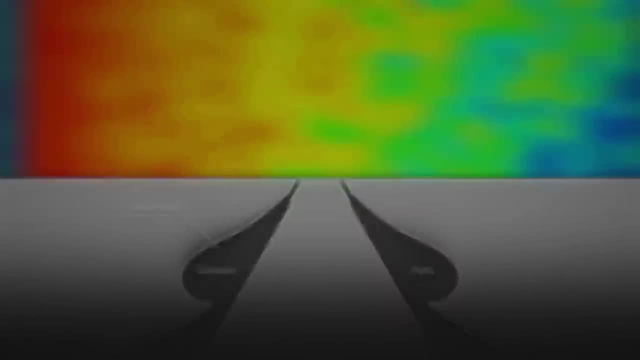 and pressure. Take the injectors: they have to be designed to handle not only high flow rates but also drastic changes in pressure and temperature. As the shockwave travels by, conditions change from 0.01 megapascals of pressure at 300 Kelvin. 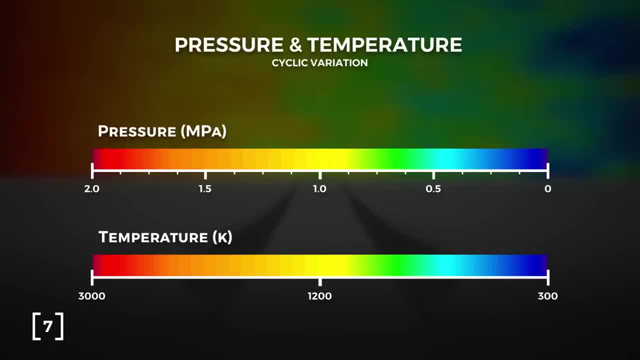 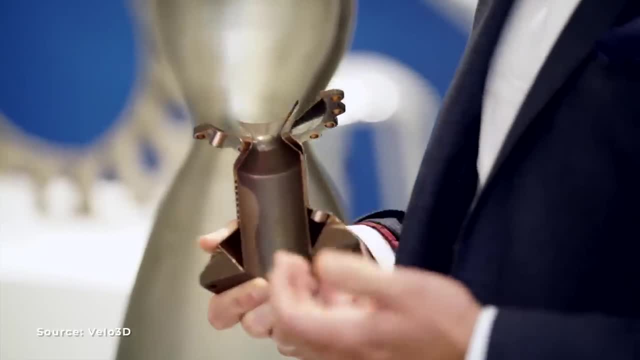 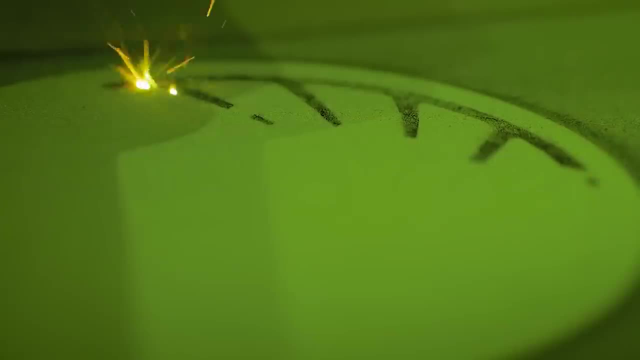 to 2 megapascals of pressure at 3000 Kelvin. That cycle happens 1000 times per second at minimum. Our copper based alloy can help us dissipate that energy, but these inlets need to switch from injecting gas to resisting the pressure of the shockwave in milliseconds. 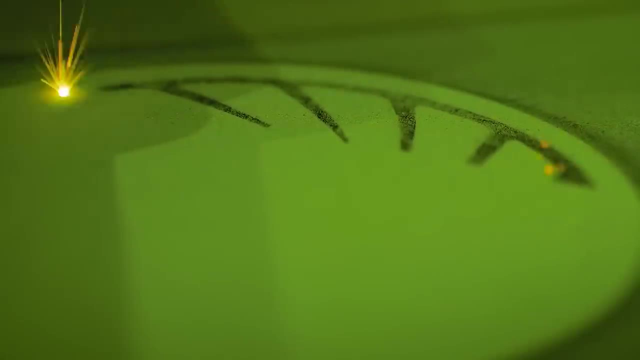 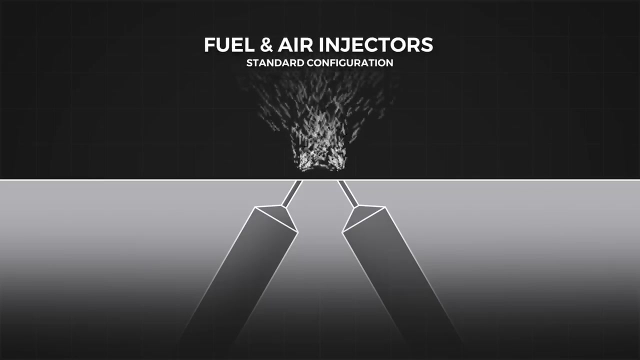 To manufacture an inlet capable of handling these conditions, the engineers needed 3D printing. A typical machined injector may look something like this, but the designers of the rotating detonation engine need to handle backflow, and for this they can turn to fluid. 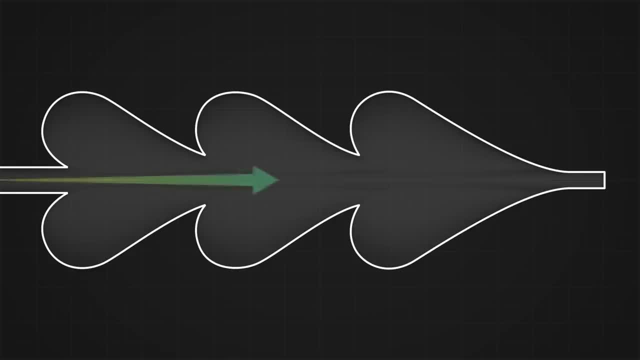 It's made of 3D printed diodes which would be impossible to manufacture with traditional cutting tools. The shape of this passage allows fuel to flow easily in one direction, but when the flow attempts to travel in the opposite direction, it impinges itself, resisting flow. 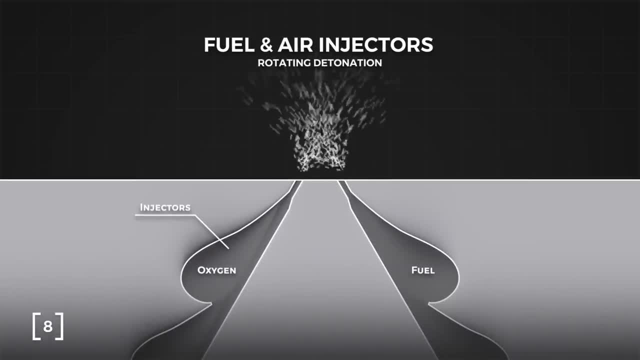 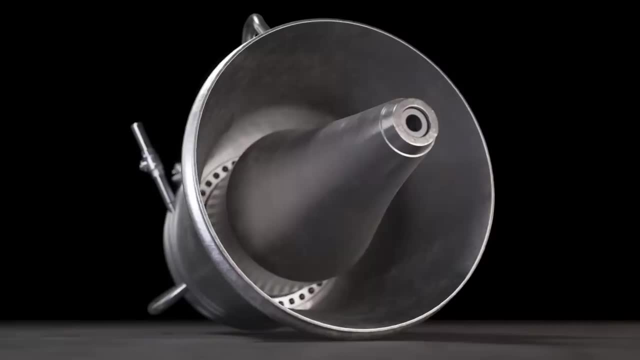 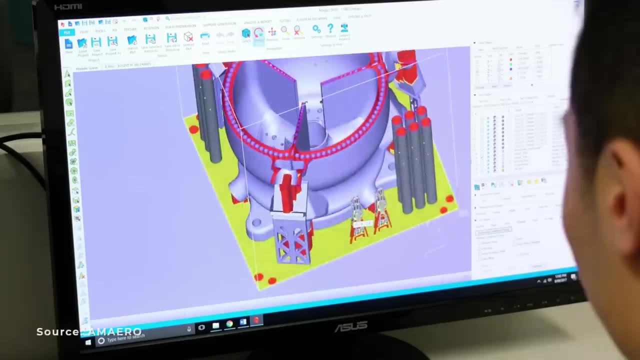 Effectively. it's a valve with no moving parts, A perfect solution for this application. The use of metal 3D printing doesn't stop at the inlet. every part of the rotating detonation engine requires delicate shaping, From the combustion chamber design to ensure the shockwave remains in rotation, to the 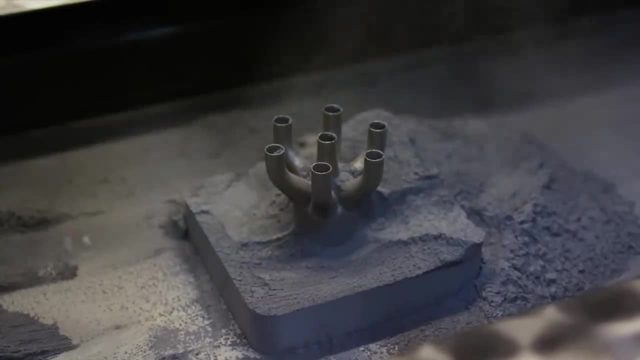 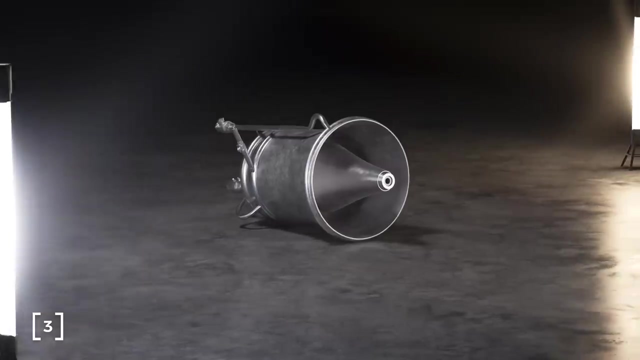 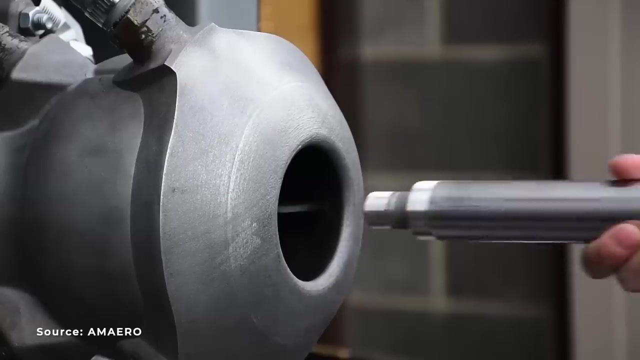 tiny cooling channels running through the walls. The rotating detonation engine that NASA developed used a 3D printed thrust chamber that was actively cooled using deionised water. It also features an aerospike nozzle. Aerospike nozzles are kind of like inside out nozzles. 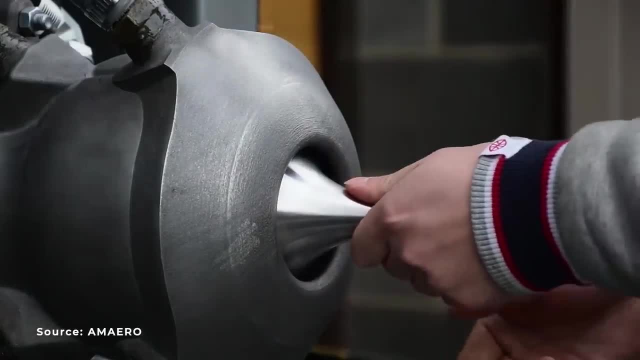 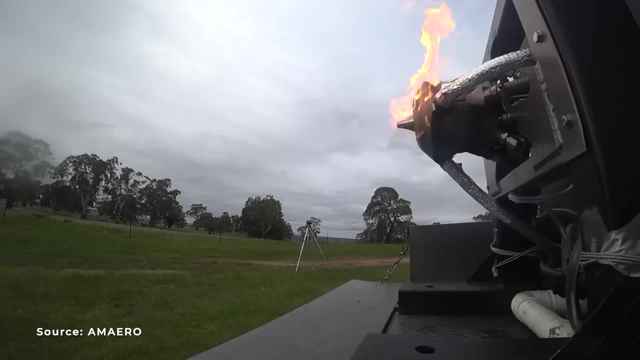 Instead of the traditional bell shaped nozzle, it features a cone at the centre of the exhaust. Aerospike nozzles allow the rocket to operate more efficiently at a range of altitudes. To understand why we need to cover some of the basics of nozzle design. 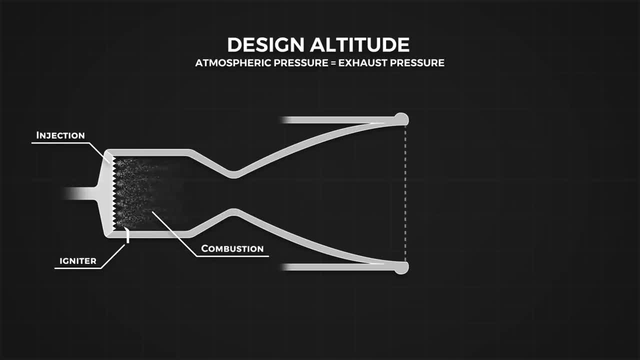 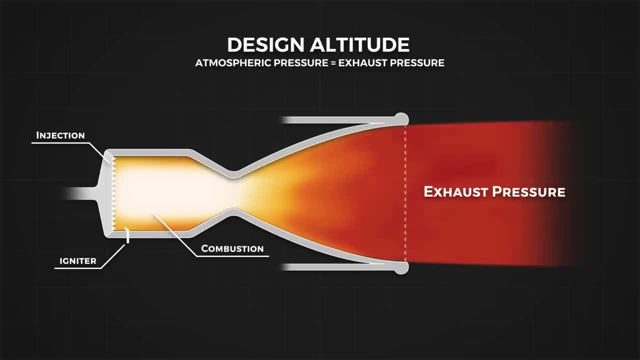 The bell nozzle operates optimally at a certain external atmospheric pressure. To work at it's most efficient, we want the exhaust pressure at the nozzle exit to equal the external atmospheric pressure. If the external pressure is higher than the exhaust exit pressure, we are operating in. 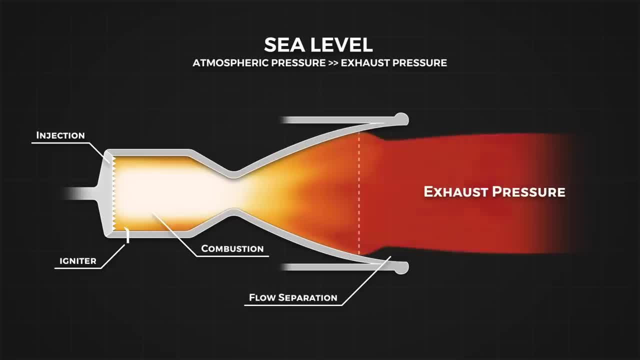 the over expanded condition, Flow separation from the nozzle occurs. The nozzle is then separated from the nozzle, The gas expands outwards outside of the nozzle and energy is lost. If the external pressure is lower than the exhaust exit pressure we are operating in. 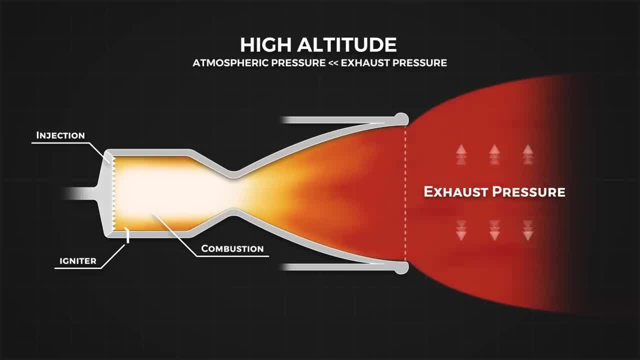 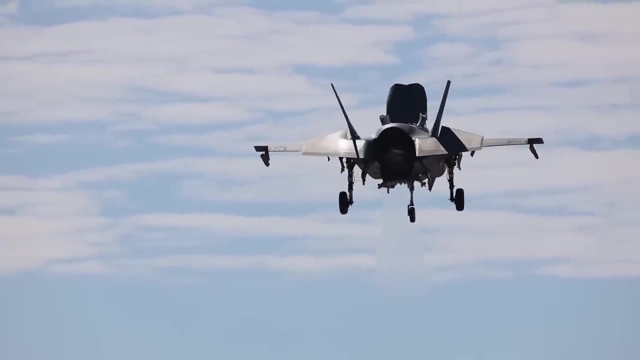 the under expanded condition, The gas expands outwards outside of the nozzle and energy is lost. However, if we match the exit pressure and atmospheric pressure, neither happen and exhaust velocity is maximised, making our engine more efficient. We could fit rockets with variable geometry nozzles like fighter jets, but this would 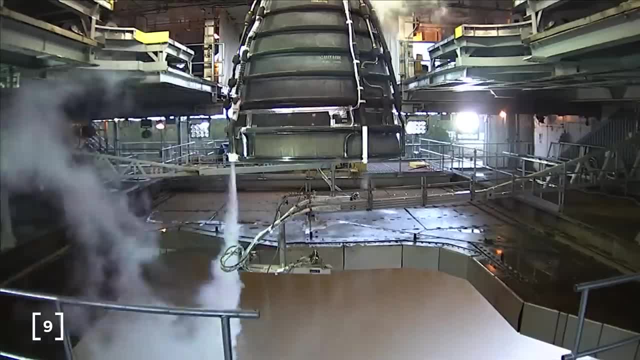 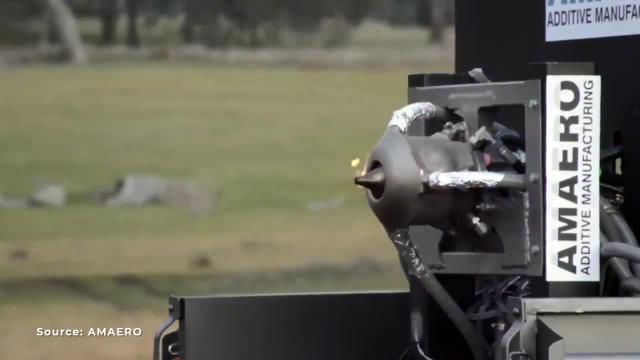 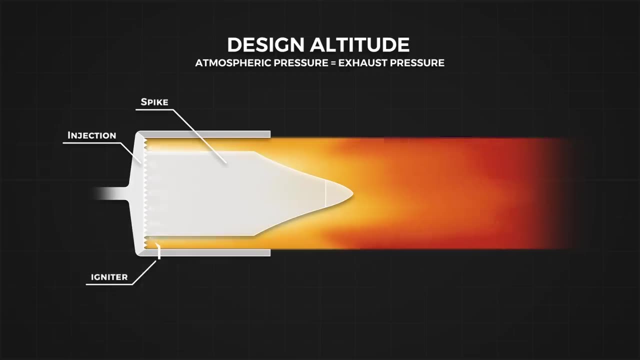 add a lot of weight, complexity and cost. These nozzles are a lot bigger than fighter jets and, until very recently, were single use. Aerospikes provide a lighter, simpler alternative to variable geometry exhausts. Here the shape of the exhaust is dictated by the external atmospheric pressure. 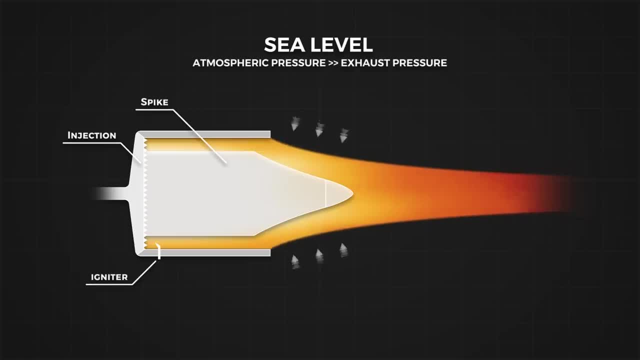 At higher pressures, at lower altitudes, the exhaust is compressed against the aerospike, which redirects the exhaust to point straight down. No flow separation can occur as the pressure is pushing it against the aerospike. As pressure lowers, the gas begins to expand. 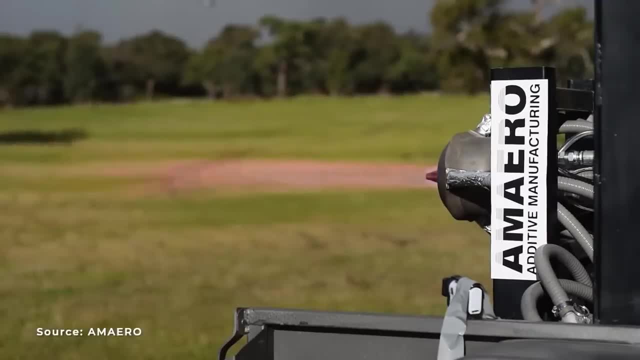 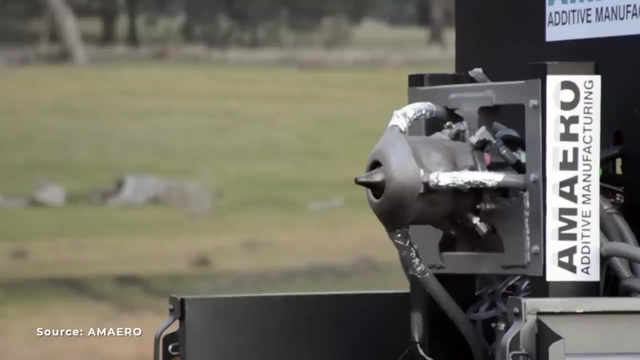 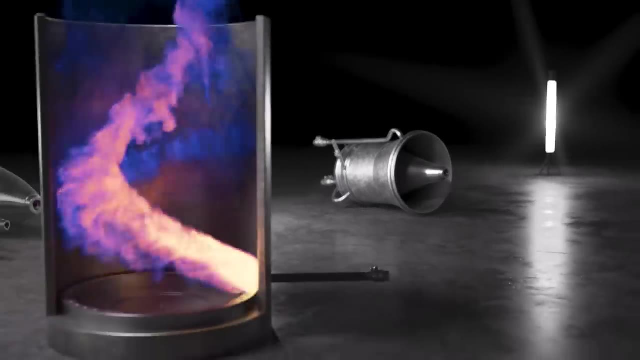 And the aerospike automatically compensates to external pressure changes. The exact science of these aerospike nozzles is a lot more complicated than this and deserve a video entirely dedicated to them alone, but the key thing to note is that they are uniquely suited to rotating detonation engines, as the aerospike engine with this cone design. 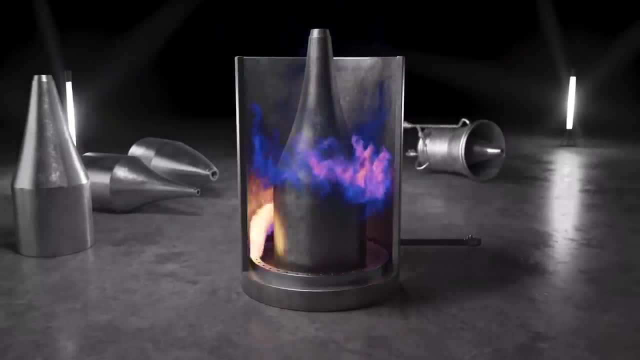 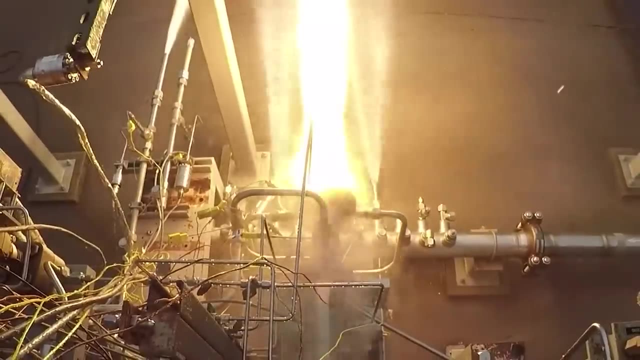 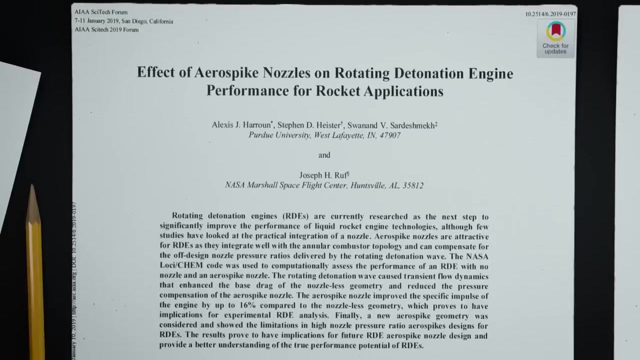 requires a circular combustion chamber, which the rotating detonation engine also requires. However, This is a more important reason To optimise the design of a bell nozzle, we need a consistent chamber pressure in order to optimise our expansion ratio. With the rotating detonation engine, the chamber pressure is constantly changing along the 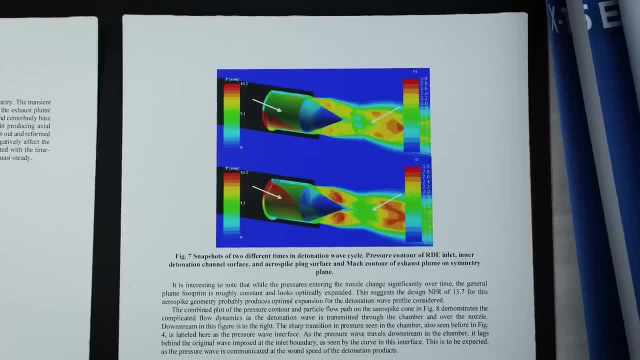 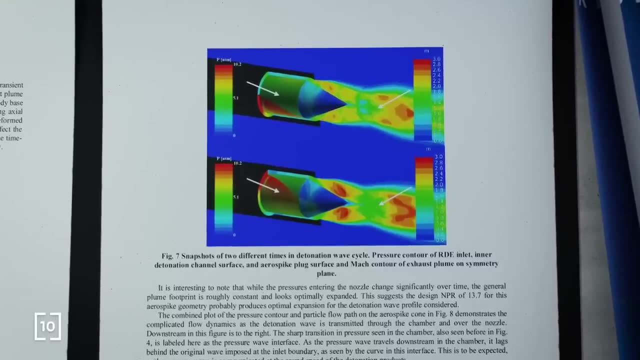 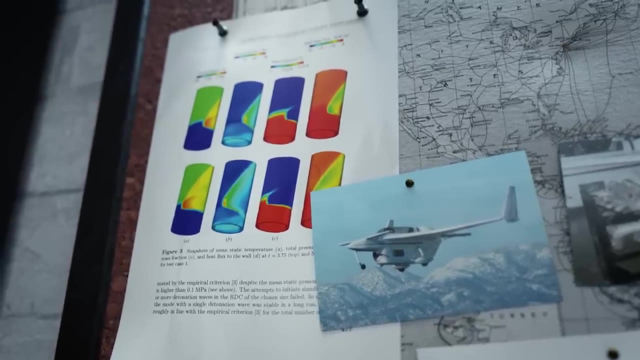 circumference of the combustion chamber. The aerospike's ability to adapt to external atmospheric pressures also help it adapt to internal chamber pressure changes. There is a lot more to do to make rotating detonation engines viable. Some prototypes, while promising, struggle to run for long enough to produce prolonged 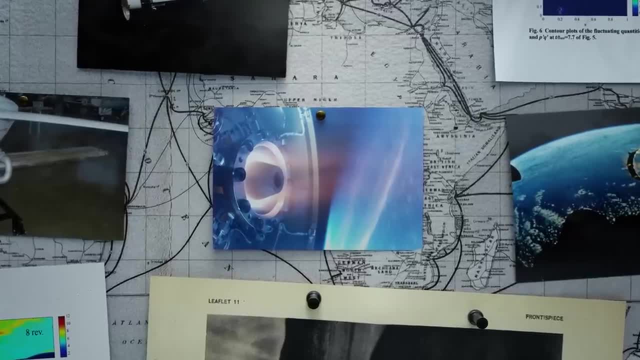 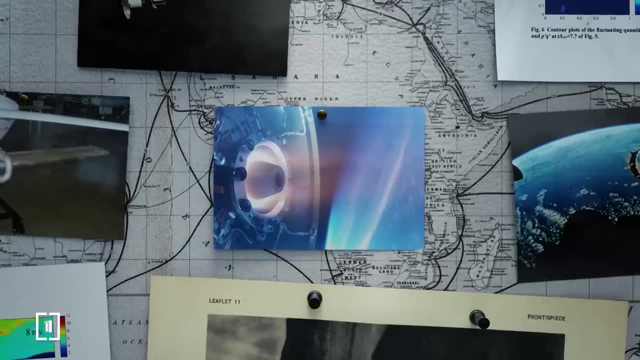 thrust. In 2021, Japan tested a rotating detonation engine in space which operated for 6 seconds, producing 500 Newtons of thrust, And while this was a proof of concept, it's a long way from the millions of Newtons traditional. 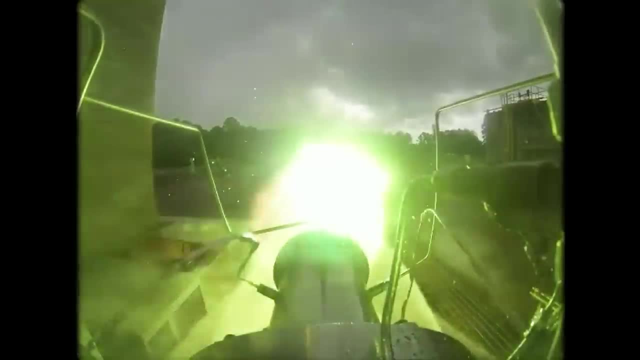 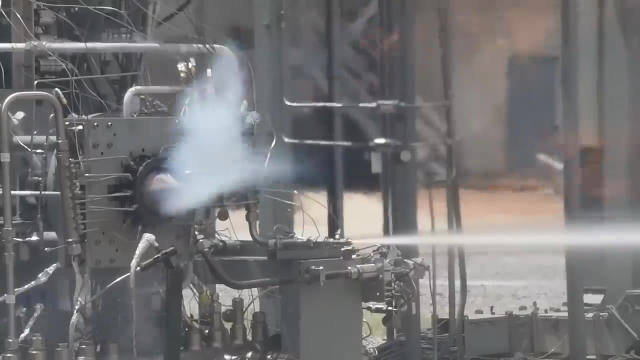 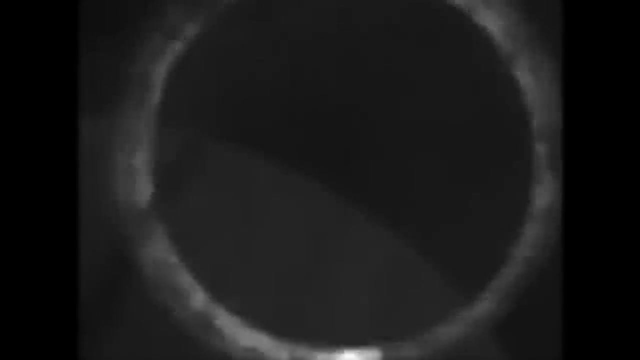 rocket engines can achieve. The mechanics of detonations are still not fully understood. This means that maintaining a stable detonation front is extremely difficult. The system is inherently chaotic. Engineers are fighting against entropy to control these powerful, turbulent flow regimes. With each revolution of the shockwave, more chaos is introduced to the system. 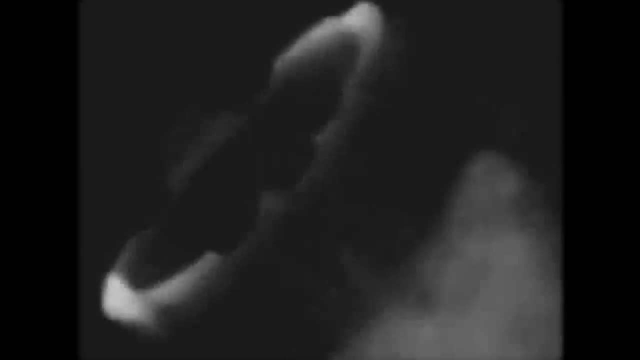 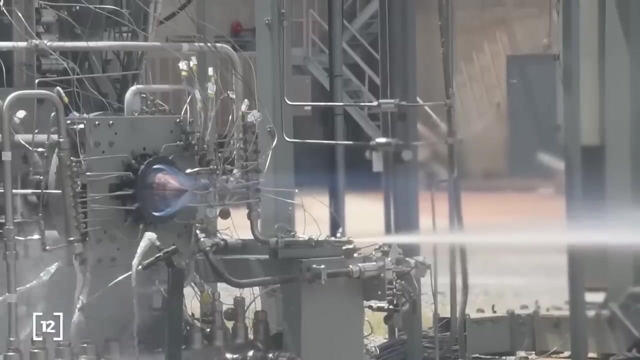 A single vortex on revolution 1 can cause a ripple effect until the rotation becomes completely unstable by rotation 20.. NASA even shared that their tests sometimes fluctuate from having 2 to 5 co-rotating detonation waves in the combustion chamber at once. 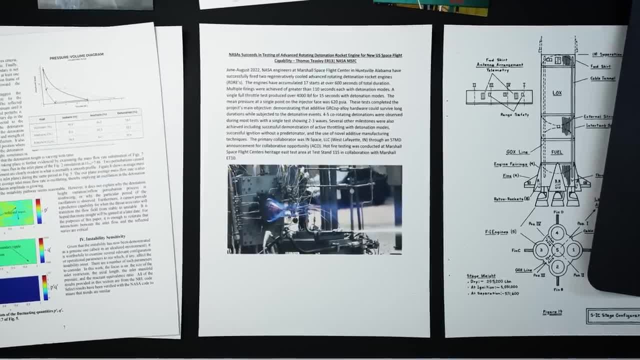 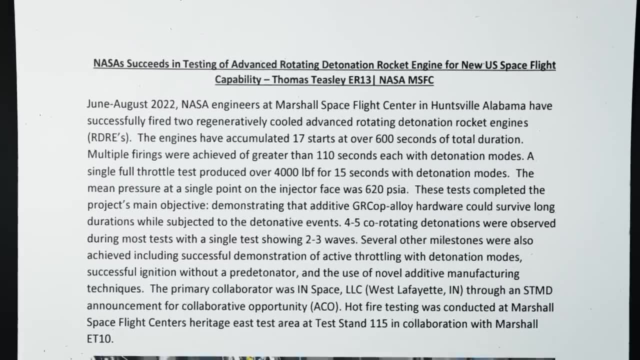 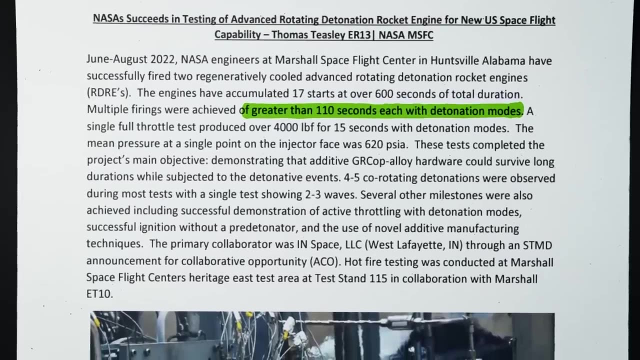 I believe it works. test was a huge milestone for the technology. They demonstrated that their copper based 3D printed material could survive for long enough in this environment, with their longest run lasting nearly 2 minutes, And they managed to successfully initiate the detonation front multiple times with. 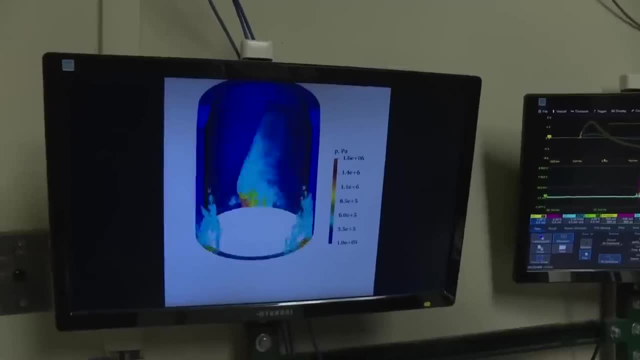 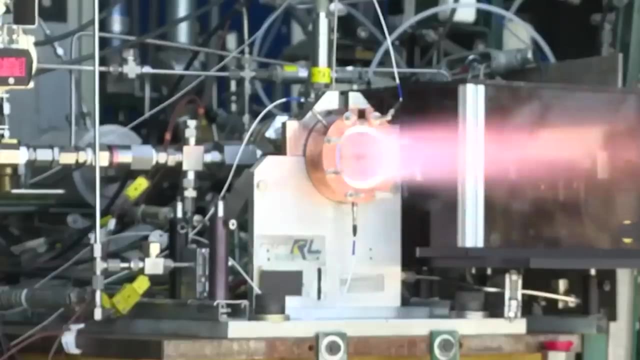 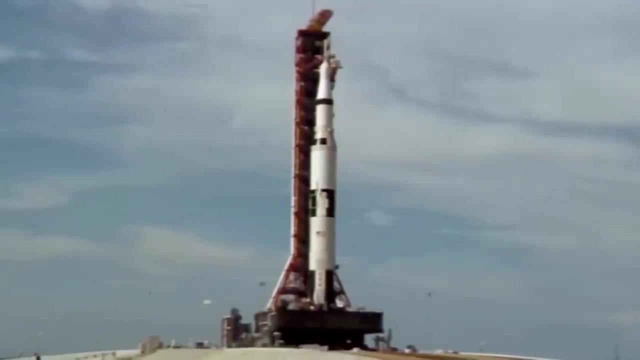 17 restarts over 600 seconds. The biggest challenge facing engineers of rotating detonation engines is creating flow models to predict these instabilities and developing methods to dampen and control these combustion instabilities, Just as the engineers of the Apollo program did all the way back in the 1960s. 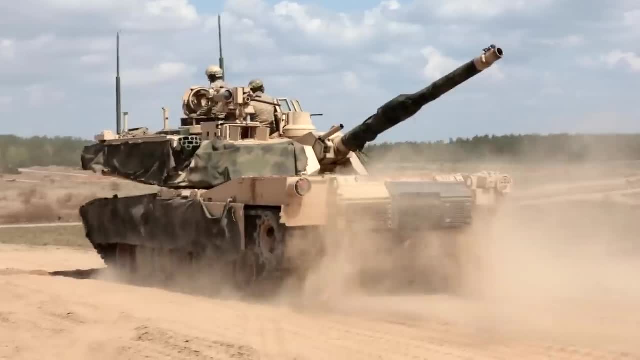 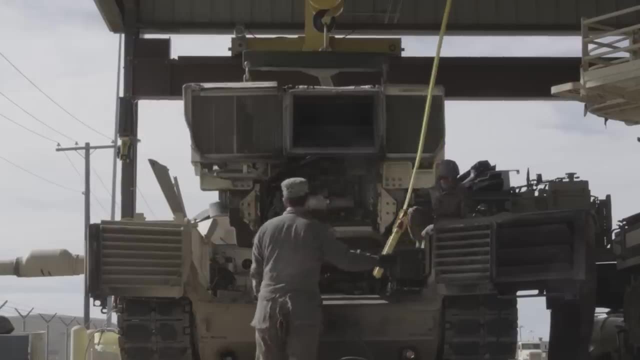 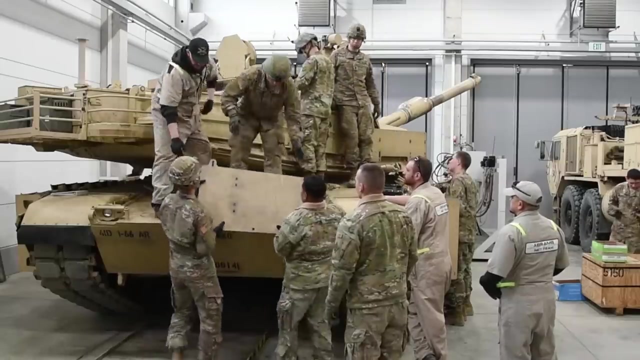 The next real engineering video is ready right now. It's about the M1 Abrams. We detail its unique turbine engine, an engine type typically used in aircraft but used in this heavily armoured vehicle for two special reasons. We dig into how the armour of the M1 has evolved over the past four decades. 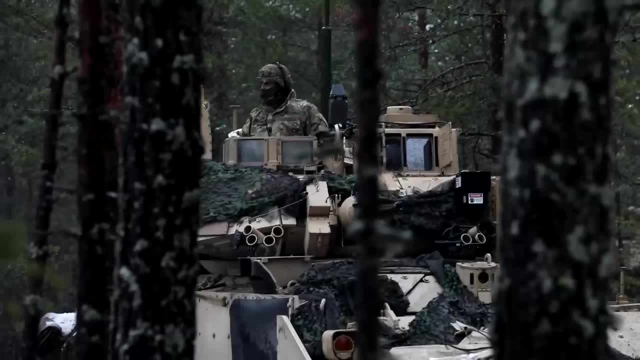 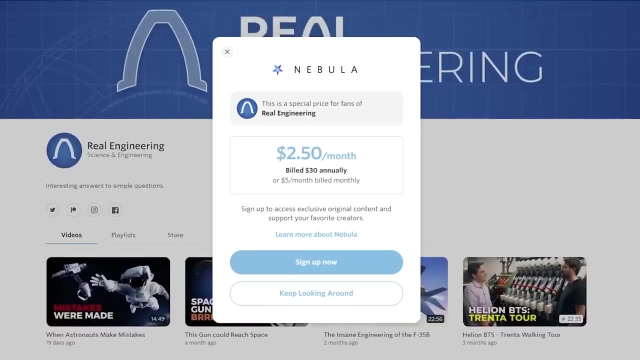 And how it works. It will be available on YouTube in two weeks, but you can watch it right now before anyone else on Nebula. as a thank you to our show's supporters, Here's a rapid fire list of incredible features you can enjoy for the low cost of just $2.50. 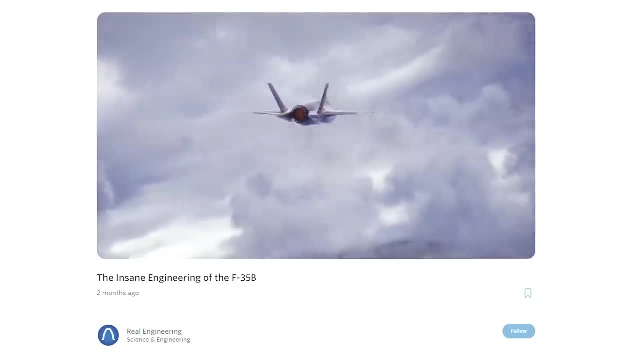 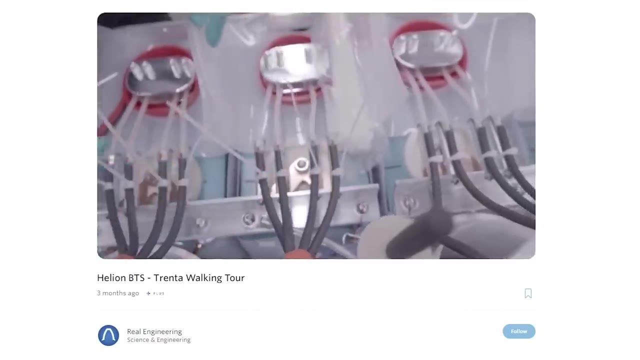 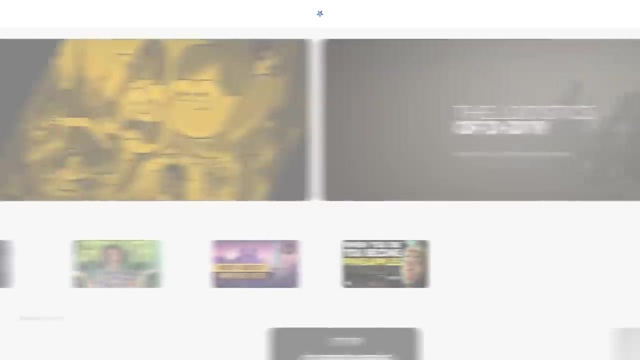 a month. Add free videos early access before anyone on YouTube. exclusive behind the scenes of our documentaries, like these two uncut interviews from our Helion documentary. exclusive classes and originals from me and all your favourite creators. I know they are your favourite because it tells me what channels my viewers watch in. 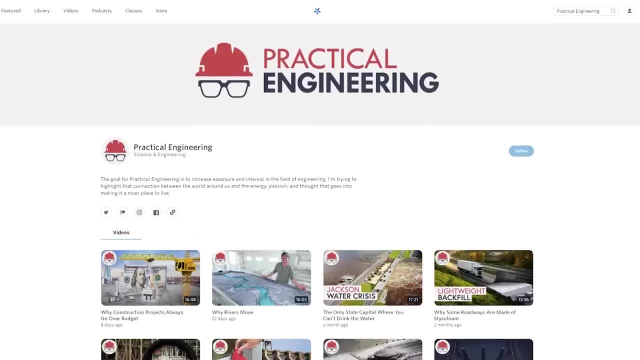 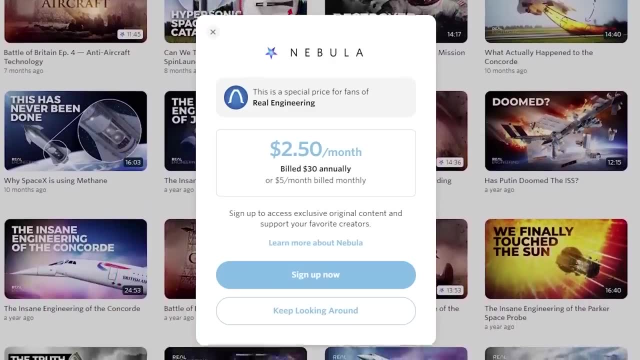 my analytics, We got Mustard Wendover Productions, Practical Engineering, the list goes on. And here's the incredible thing: By signing up with my link, you aren't just supporting me, You are supporting educational creators across the board, Because we all own a percentage of this platform. 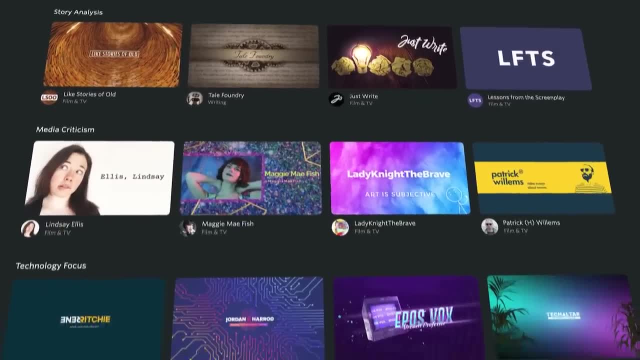 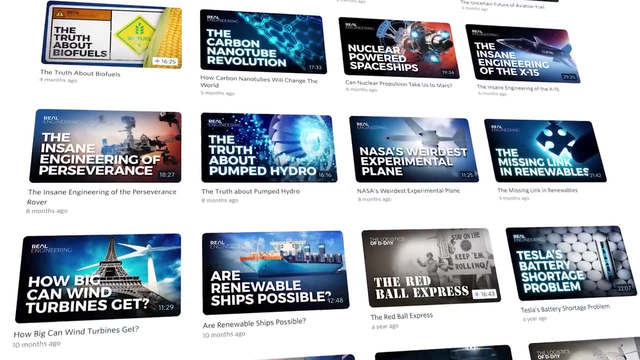 We created it to give us creative freedom, and we've achieved that. Nebula is the lifeblood of our channel. As sponsors and ad revenues have dropped lately, Nebula is what is ensuring our incredible team of writers, animators and editors across. 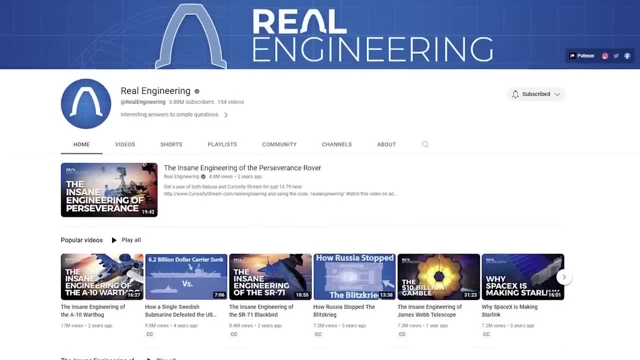 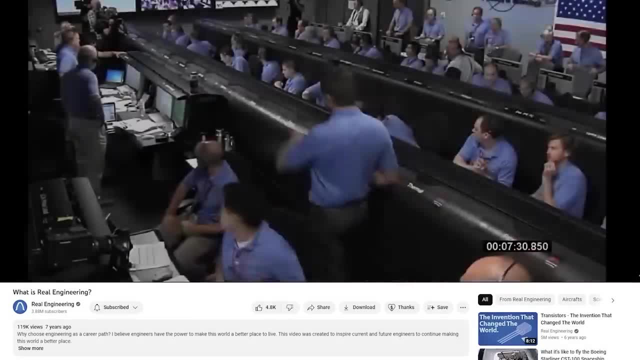 real engineering and real science, including myself, can feel secure in uncertain financial times, And that's thanks to you. Real engineering started with just me. I barely knew how to animate. I had a dream of recreating the magic I felt watching nature documentaries on TV growing. 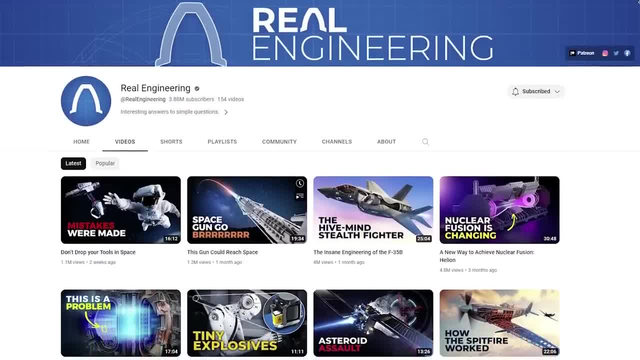 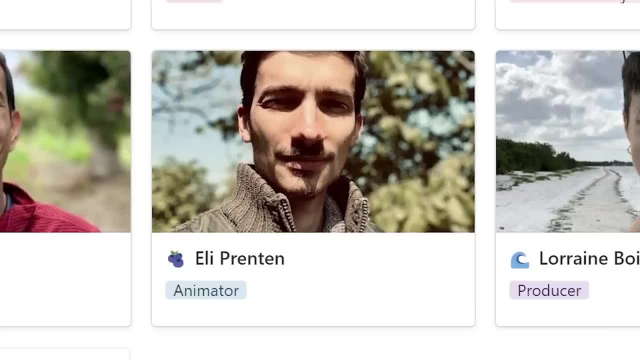 up, but for engineering. Over the past six years, I've continually reinvested revenue to hire the incredible people that make this channel possible. My name is Nebula Mike Dylan, Stephanie Eli Kirtan, Lorraine Josie Graham.